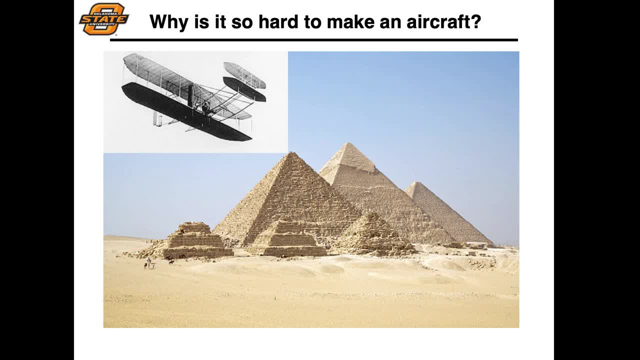 Now you could really look at this from a standpoint of kind of comparing it to traditional structural design, design of buildings, for example, bridges and the like, And of course we've been doing this not only for centuries but Obviously for millennia. in structural design of buildings, as usually emphasized on very, very high safety factors and safety margins, such that a typical building will be able to carry much greater than its actual design load. 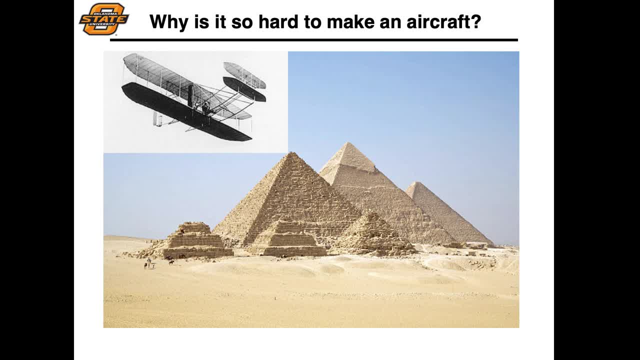 Now, one of the things that makes aircraft design so difficult is the structural requirements for an aircraft design And to be successful not only in terms of being profitable or being efficient, but just being structurally sound- are very, very small, So you don't have a lot of margin for error. 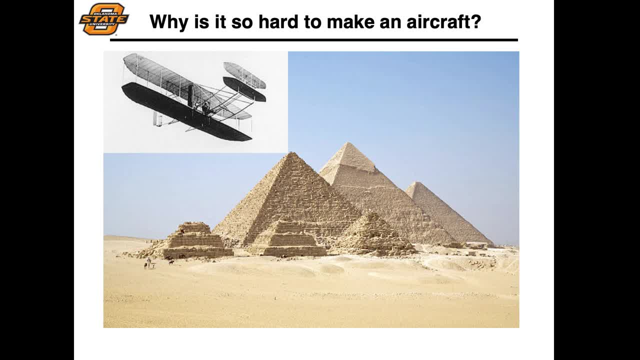 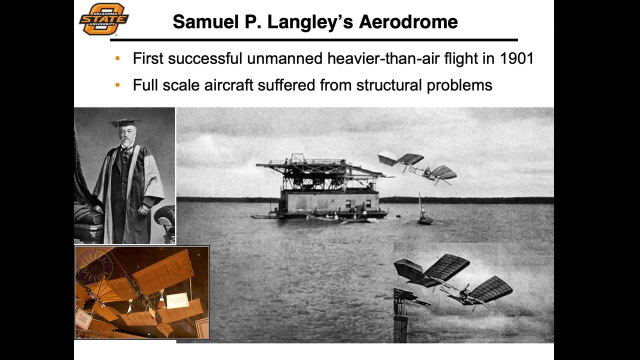 If you end up making your aircraft too heavy, it's not going to fly. However, if you make the structural design too weak in order to try to lighten your aircraft, then your aircraft is going to fail, And this is really exhibited through a number of historic failures, and we'll give a couple of examples of these throughout the 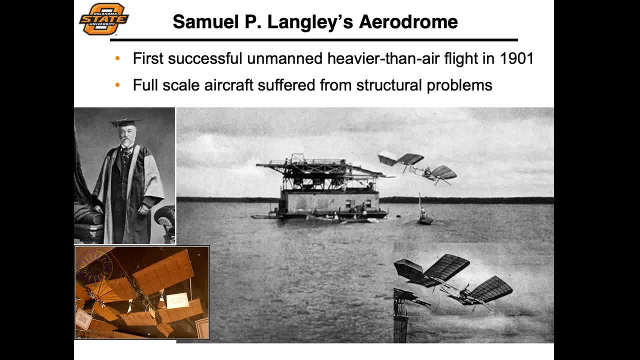 lecture. But really, you know, one of the earliest of these is Samuel Langley's aerodrome And, as we mentioned earlier in the semester, Samuel Langley, who was the secretary of the Smithsonian at the time, is actually credited with the first successful unmanned heavier-than-air flight in 1901.. 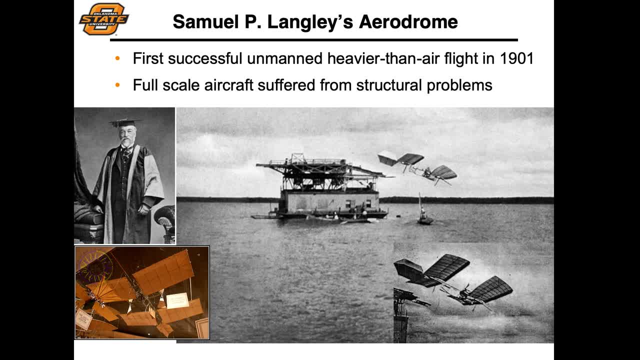 And of course this was part of his goal to be able to have a manned heavier-than-air aircraft development, And he tested this system, which he had scaled up from his unmanned flight, literally weeks before the Wright brothers flew. He actually had a pretty sound aerodynamic design. 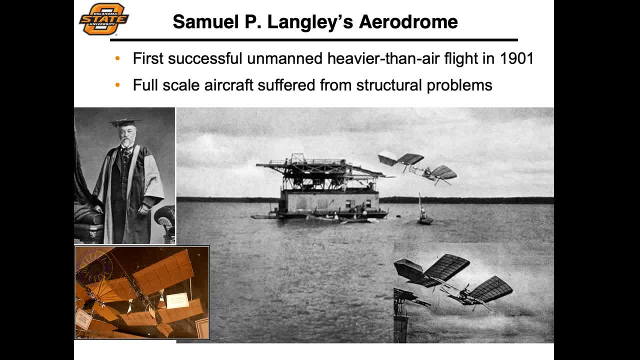 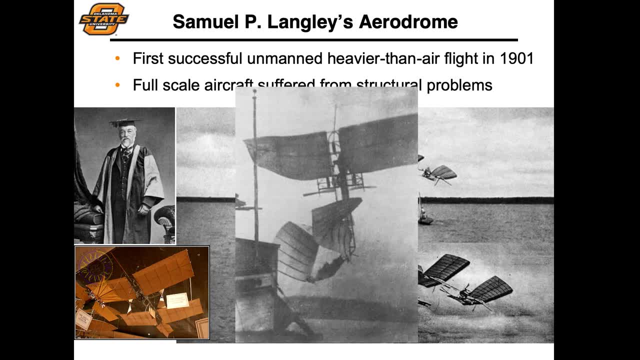 He had an excellent propulsion system, but he was deficient in his structural design, almost resulting in the death of the pilot, And really the issue was that he just wasn't sufficient in terms of scaling up the structural design requirements as he moved from the smaller prototype aircraft. 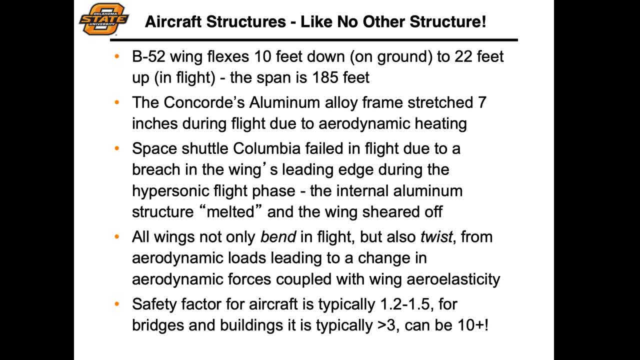 to the full-scale aircraft. Now there are a number of examples that you can point to throughout the aviation industry that really give some kind of amazing conceptual realization, And I think that's a really good example of how unique aircraft structures are. For example, the B-52 wing flexes a total of 32 feet from 10 feet down when it's resting on the. 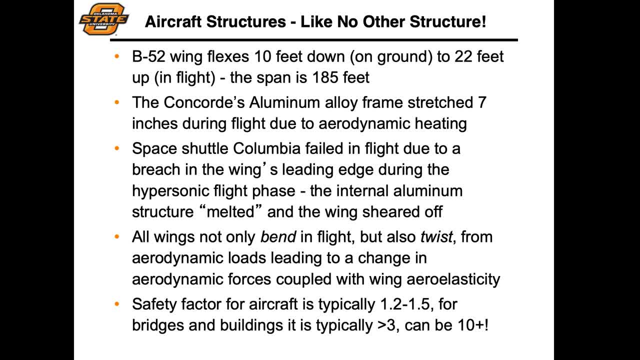 ground to 22 feet up in flight, And so, if you think about this, 32 feet is a function of the overall 185-foot span, And that's a substantial fraction that this structure is flexing. The Concorde, when it was in operation, actually stretched seven inches during flight just due to. 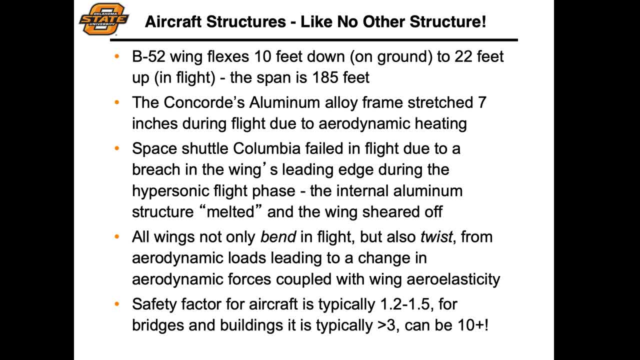 aerodynamic heating. So you know it grew over half a foot as it was flying. And the Space Shuttle Columbia. if you look at really both the accidents of both Space Shuttle tragedies, you know it was really structural failures, you know that led to both of these. So the Space Shuttle Columbia, 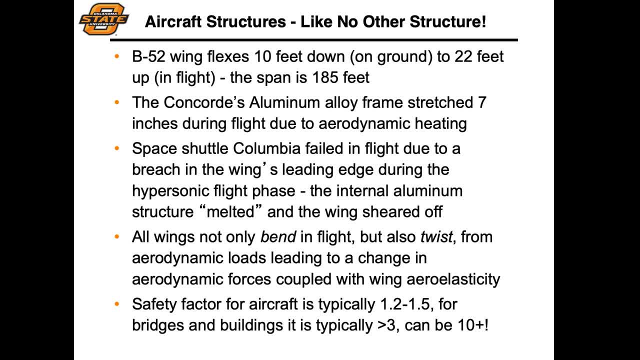 specifically, you know, failed to fly, And so you know, the Space Shuttle Columbia, you know, failed during flight as it was re-entering the Earth's atmosphere, due to an accident during the ascent phase, when part of the insulating foam that covered the main external tank broke off. 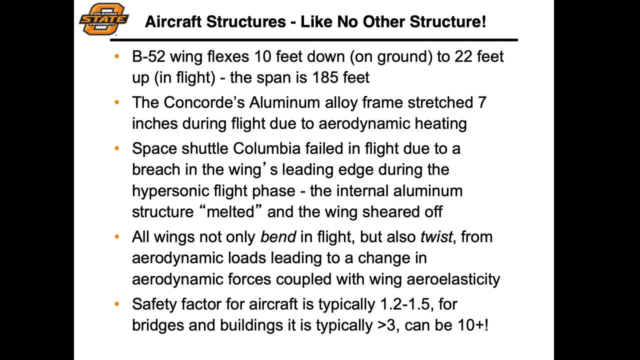 and ruptured the carbon-carbon leading edge And, as it was re-entering the Earth's atmosphere, the heating, the ionized gas, the plasma in the atmosphere, due to the high speeds as it was re-entering- at Mach 25, actually entered that internal structure and melted. 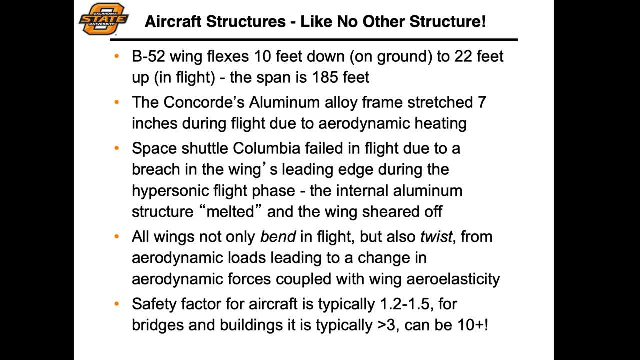 the interior of the supporting structure that held the wing on. Now, as we'll see from examples, all wings bend to some degree in flight, but most of them also twist as well. So as the wings are undergoing aerodynamic loads, we don't expect them to be static. So there is going to be some. 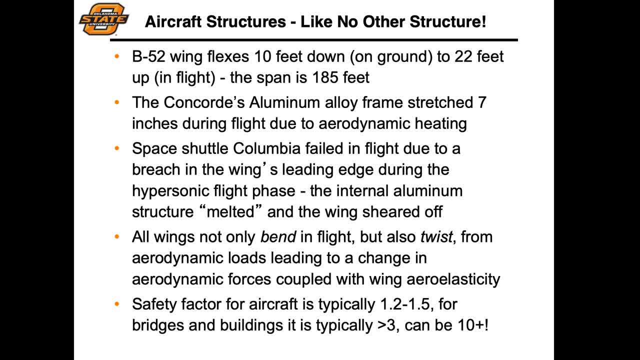 changes in deformation as you have the aerodynamic forces acting on the wing. We'll talk a little bit about aeroelasticity but, as we'll see, that's, you know, really even too complicated to cover in, you know, next semester's Structures course at the undergraduate level. 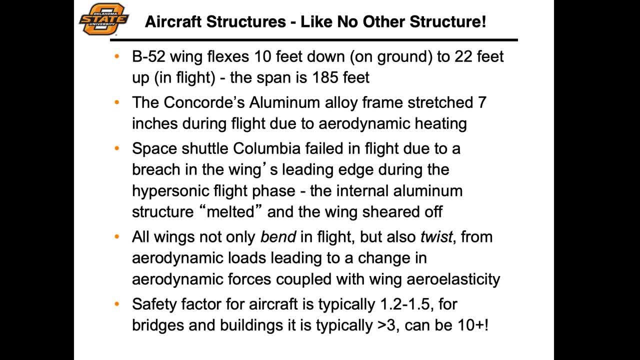 Now, as we mentioned on the previous slide, safety factors for bridges and other buildings, you know, can be very, very high, you know, sometimes really an order of magnitude greater than the design load. But well, for an aircraft, however, you'll typically see, 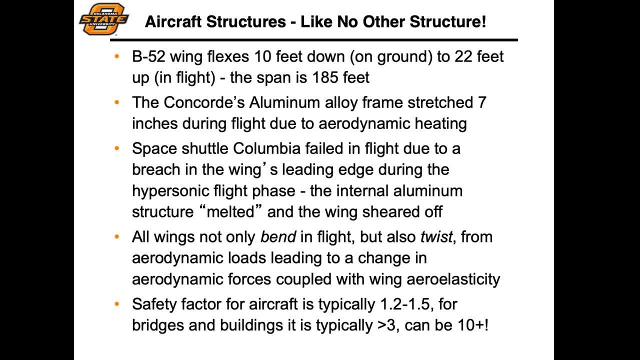 that your safety factors are on the order of about 1.2 to 1.5, the maximum design loads that you expect to see in flight. So you have a relatively small margin, of say, 25% to 50%. 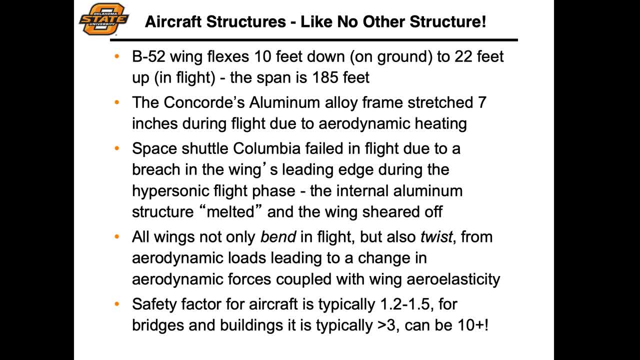 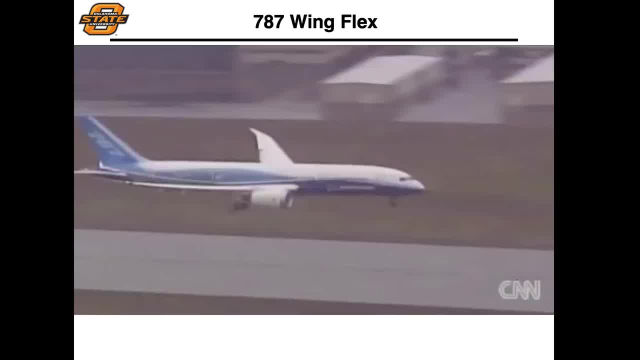 where you might see some failure in some component of your aircraft due to structural limitations. Now here's an example. Here's an example of the Boeing 787 coming in on a landing. So, as it's approaching its landing, again we can assume that this is a quasi-steady state attitude that it's in. So, even though it's. 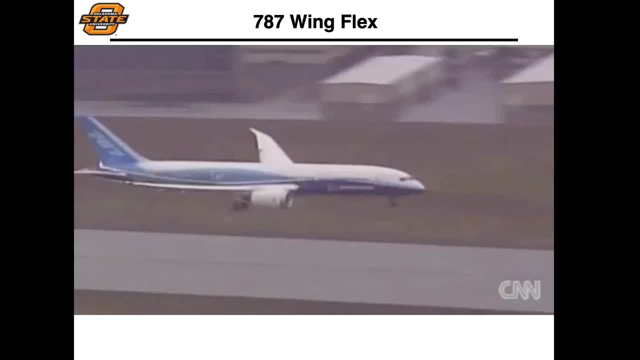 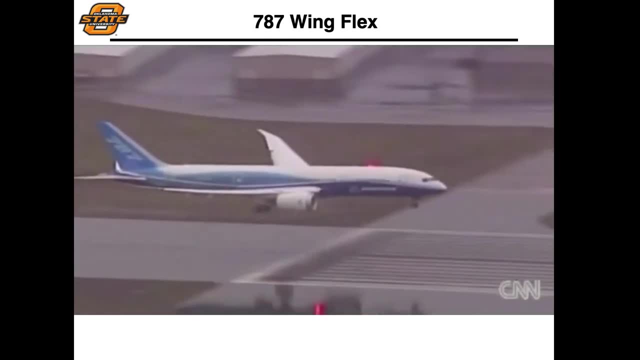 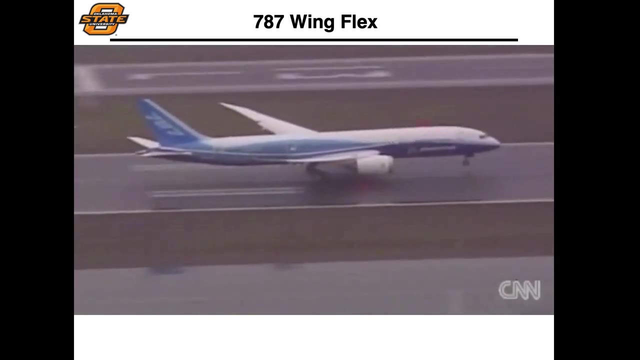 descending. that's a relatively slow flight. So again, it's more or less in level and steady flight. So we expect lift to be equal to weight in this scenario. But watch the wings as it goes through the wings. So as the wings are unloaded you'll see the wings go to their- you know- static. 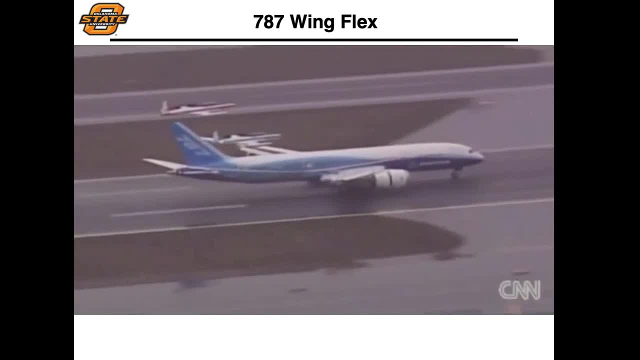 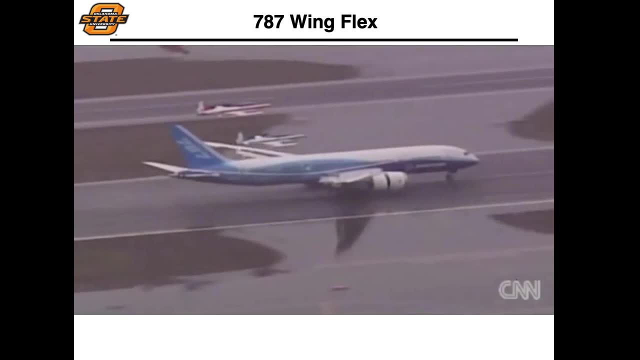 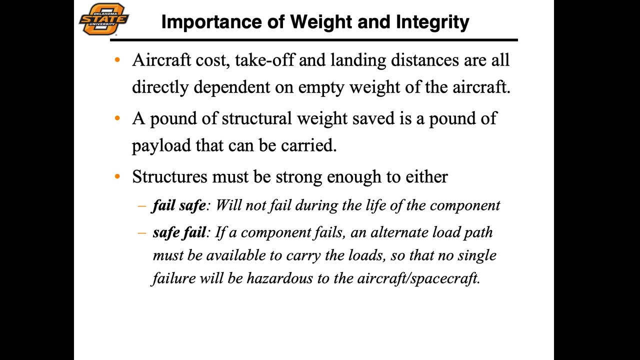 unloaded position, You can see the amount of flex that you had in those wings as it goes from the loaded to the unloaded portion of the flight. Now there are really very important design considerations that we have to take into account when we're looking at a flight. So let's take a look. 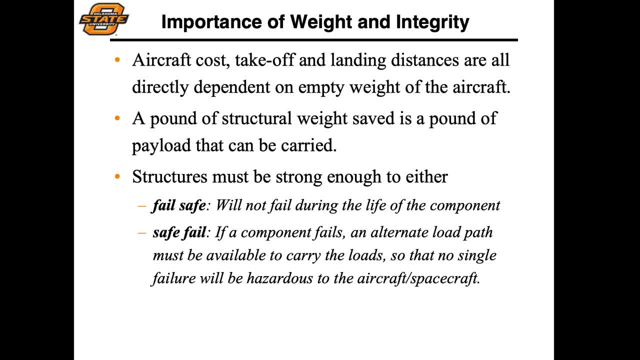 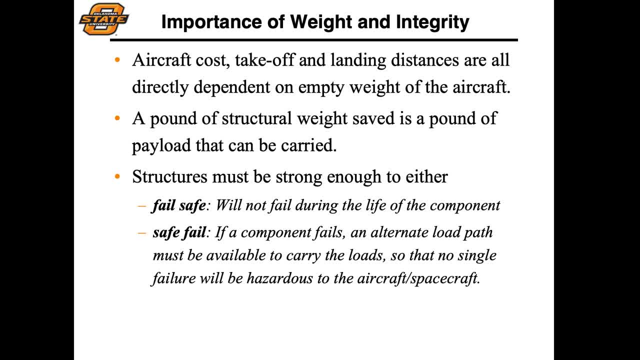 so, first the aircraft cost and then things such as take off and landing distances, which are going to determine your runway considerations and the type of airport that you're going to be landing at, are all directly dependent upon the empty weight of the aircraft. 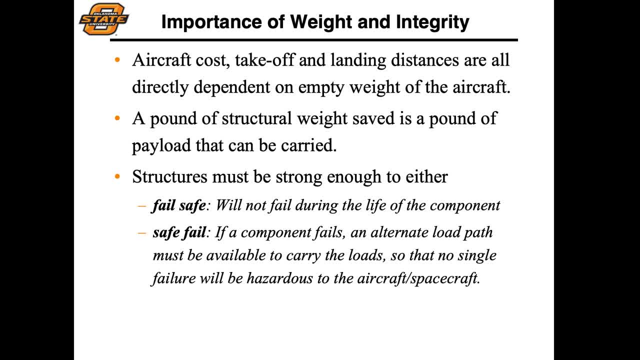 So that's going to be conducted not only mandated by things such as the FARs, but really driven by basic design considerations. as your aircraft gets larger and uses more material, that cost is going to go up, and what we'll typically see is that saving pounds on an 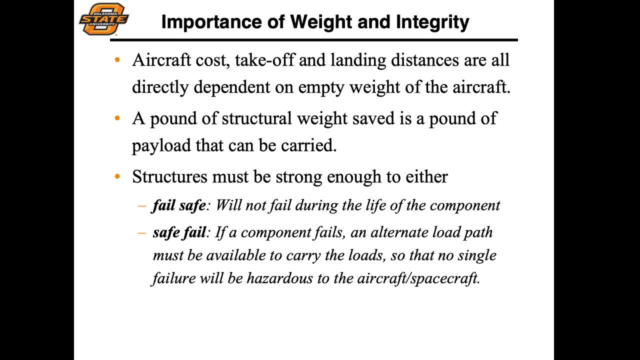 aircraft can maybe save thousands and tens of thousands of dollars per pound on the overall cost of the aircraft- and we'll talk about this in another lecture, specifically discussing weight prediction and considerations. So you can also think about this from the standpoint of how much payload that aircraft is going to be able to carry If you can save a pound of structural weight. 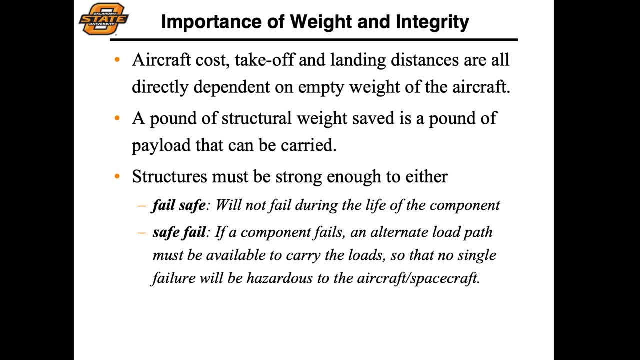 while still maintaining the same load carrying capability of the aircraft. that means that you can then carry a pound of payload instead, or perhaps a pound of fuel if you have the volume to carry that fuel as well. So obviously, driving that weight down is going to be able to make your aircraft more. 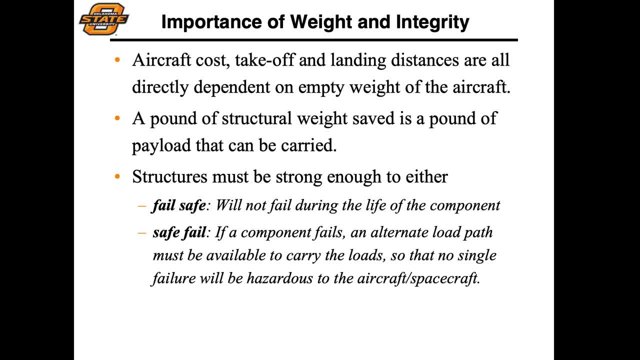 effective and possibly more profitable as well. Now we also have to think about the philosophy around our design considerations for our aircraft, how we're designing this and typically what we're going to do is we're going to think about the philosophy around our design considerations. what we do not do is design around a fail-safe philosophy, meaning that those components will 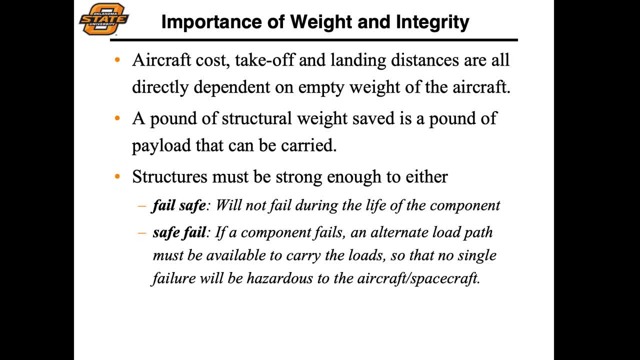 not fail during the life of operation or, you know, before those components are replaced, and that is usually due to the fact that that requires a very high weight safety of factor and that ends up just becoming more costly, Since we've done a lot of process testing to see what you can afford in an aircraft. so what we tend 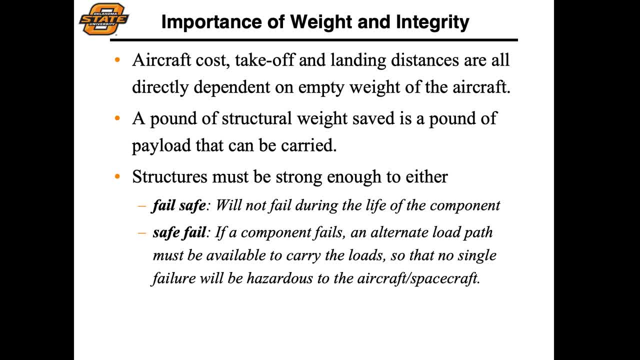 to do is take an alternative process, which is instead of fail-safe. we have a safe fail procedure where, if a component fails, there is some alternative load path that is able to carry those loads. so that way, no single failure will be hazardous to the aircraft that we're designing Now. obviously there. 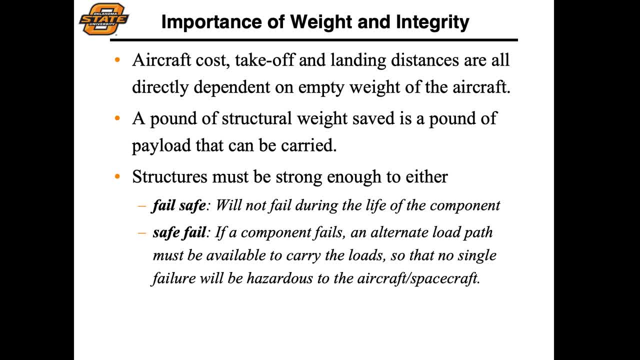 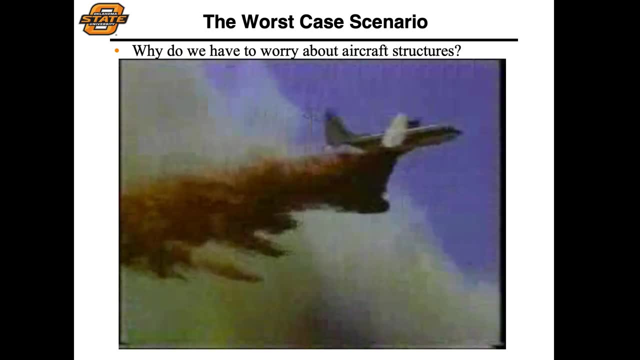 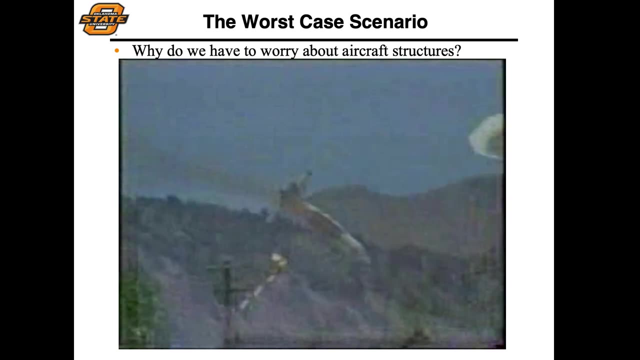 If we have a certain component fail on an aircraft, we can't get around it. So we just want to make sure that those cases are very few and far between. So here's an example kind of the worst case scenario, where we have a converted C-130 that's being designed for a really strenuous type of mission. 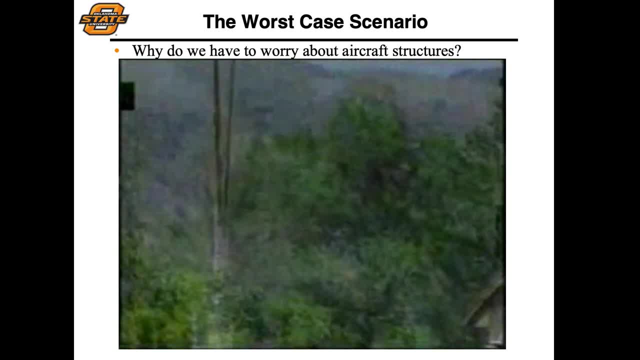 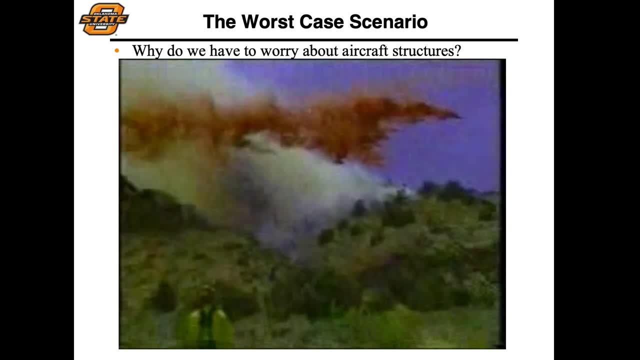 And we'll talk about this in a few minutes. when we look at the actual load that's being carried on these types of systems, You'll see here as it's executing a high G maneuver, in this case going through a pull-up maneuver. 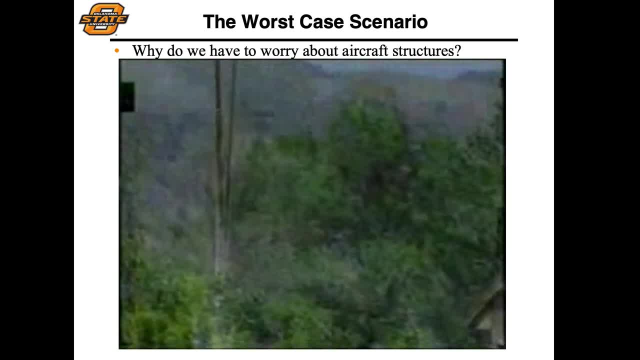 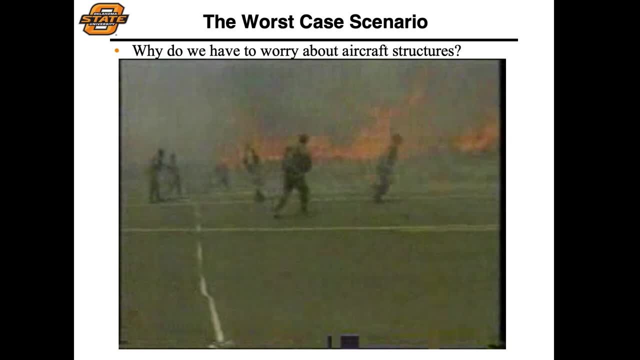 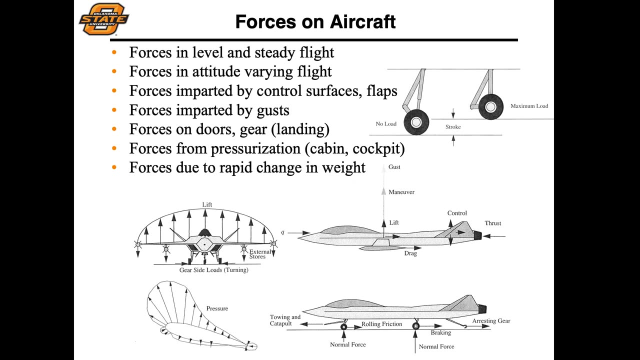 as it's preparing to deploy its fire-retardant payload, that the wings fail and essentially break off, resulting in total loss of the aircraft and all of it. Now, as we mentioned previously, a lot of the forces that we see on the aircraft are primarily due to unsteady loads. 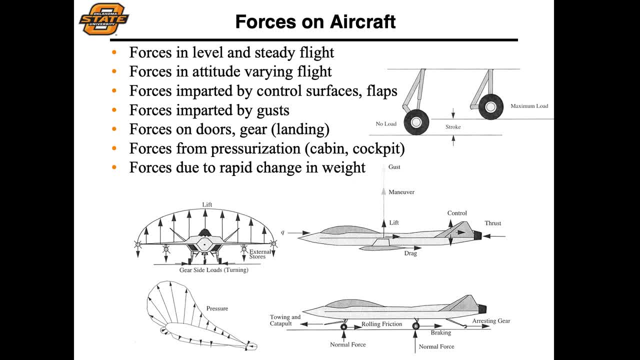 So, even though we'll be thinking about that on-design consideration, that's really the lowest and the minimal types of loads that we're going to see acting on our aircraft. So almost always design from the structural standpoint of their aircraft around unsteady or dynamism. 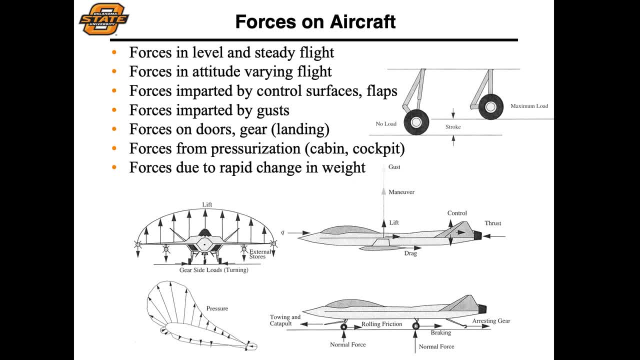 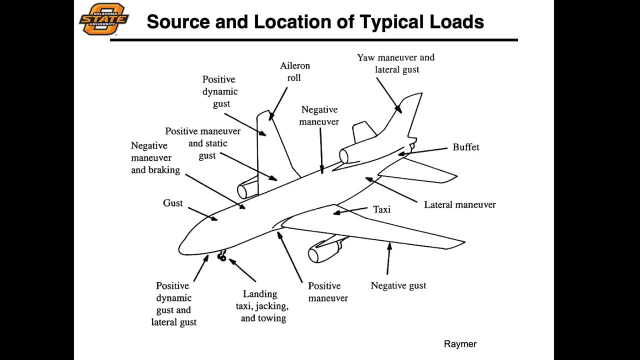 Meaning we are going to look at those, those dynamic forces acting on an aircraft, because those are going to be the most stringent loads that we're going to see for our aircraft acting during flight. So those loads are going to be acting on various places across our aircraft. 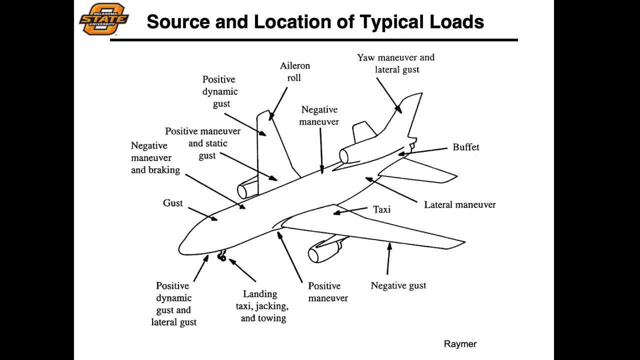 so we can think about, you know, wings as one example, But we'll also have to design the arpenage, the fuselage. loads acting on individual elements, such as landing gear, are transferred throughout the rest of the aircraft, because any load that's going to be acting at one part of the aircraft is really 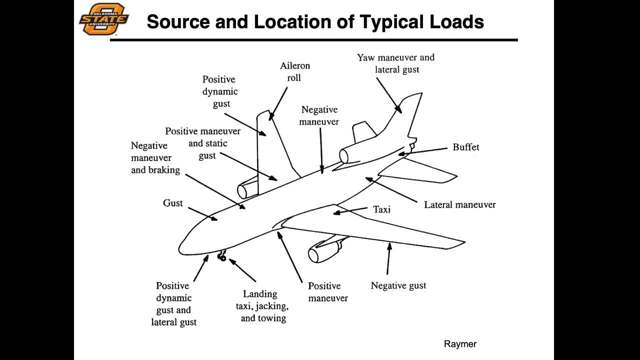 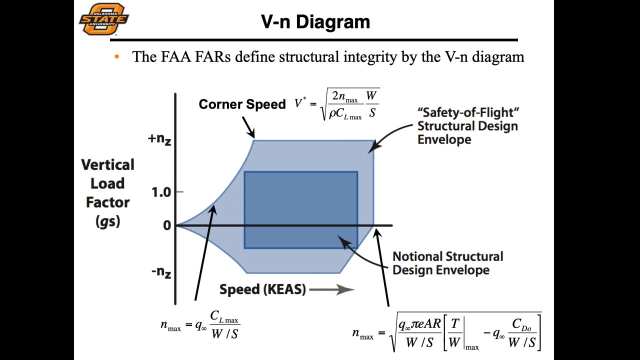 going to affect the entire aircraft as well, so we have to think about the load paths and how those loads are actually being translated or transferred from one part of the aircraft to another part of the aircraft. now, of course, this has a big impact on what our vn diagram is going to look like. 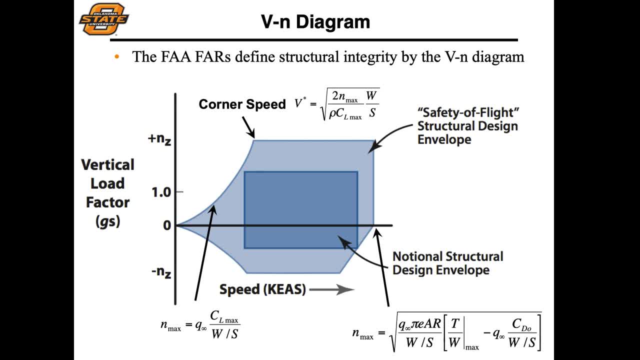 because, as we said before, this is really a structural flight envelope for our aircraft, that vertical axis that determines what our load factor capabilities are. we usually use this as a design requirement. so, for example, we might have a maximum load factor of 2.5. that's mandated by 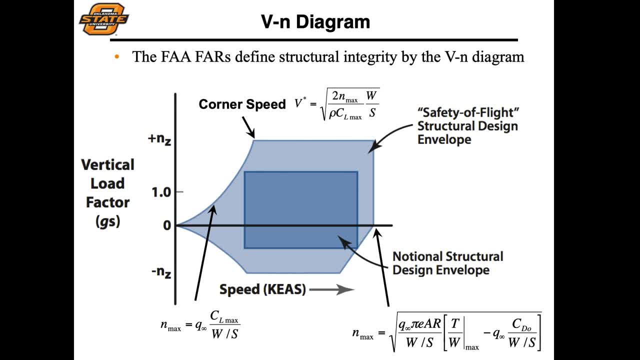 the far you on our particular aircraft design and in that case then we have to design the structure around those loads in mind. now there are many cases where aircraft are going to see you know loads kind of outside of uh, you know potential normal operating loads. and here's an. 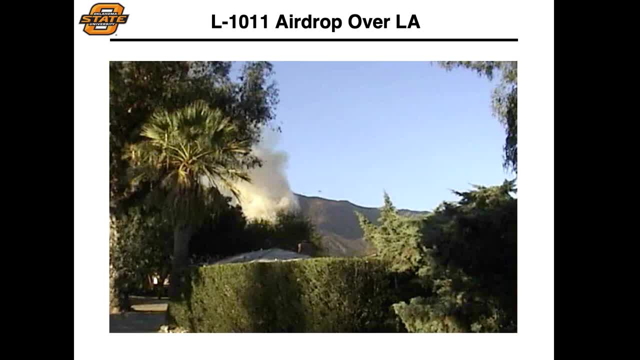 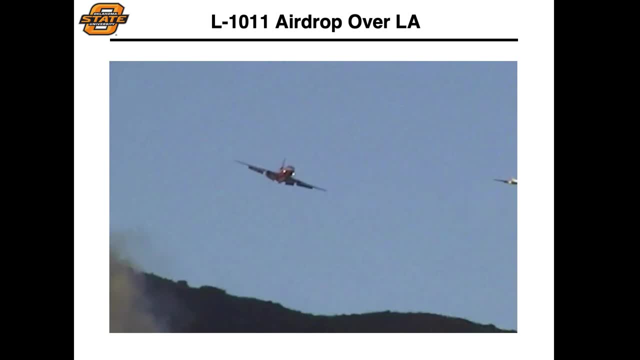 example of an l1011- this is another airdrop, in this case particularly over la- and think about what this aircraft is going to be doing in that case. we have to design the structure around those loads and we can also say, look, if this aircraft is going to be using some kind of 차� or a. so we're not actually going to be making any kind of operations out of this aircraft, because that's not a good idea, but again, we're going to have to consider what these aircraft is doing. i don't know how much you know payload is carrying in terms of the fire retardant, but it's not in common for you know these converted aircraft to carry around 10 000 gallons. so you're talking, you know, somewhere on the order of 50 000 of potentially 70 000 pounds worth of payload being deployed in a very, very short period of time. and so you'll notice that, as this aircraft is actually maneuvering, 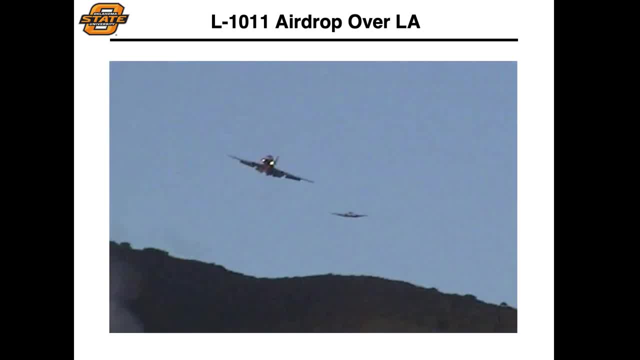 being deployed in a very, very short period of time, and so you'll notice that, as this aircraft is actually maneuvering, watch how the aircraft starts to dive as it's deploying its payload, and really what it's doing here in this case is it's changing its attitude, because, as it's deploying its payload, the dynamic 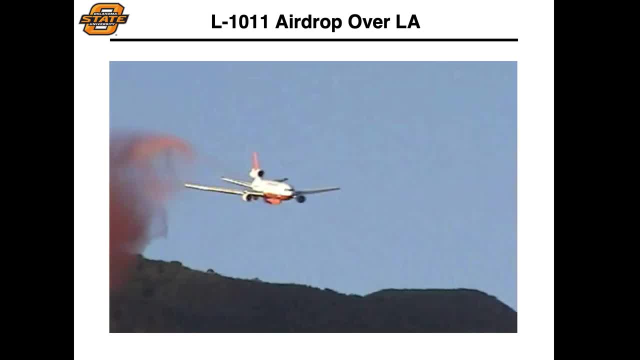 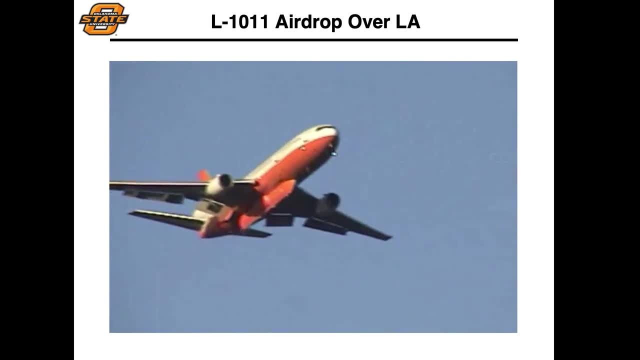 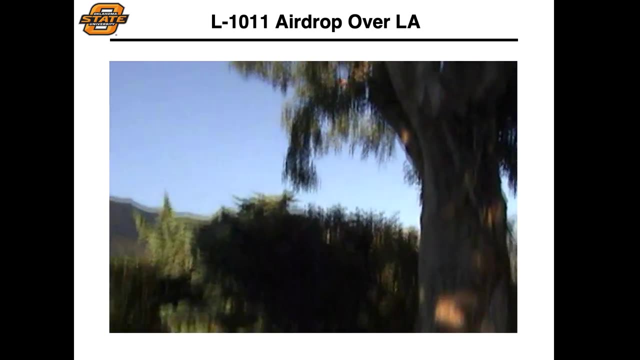 load on the aircraft is changing, the aircraft is getting lighter and you know again, ostensibly the nominal condition here is that the lift is going to be approximately equal to the weight of the aircraft and if you're deploying a massive amount of load, in this case a significant fraction. 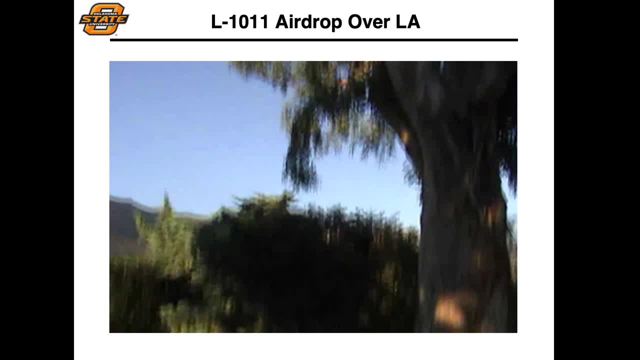 of the overall maximum weight of the aircraft. you have to be changing the lift at the same time that you're actually deploying this load, so think about what the wings are undergoing as it performs this payload drop and simultaneous maneuver. so, as part of that, the structural design. 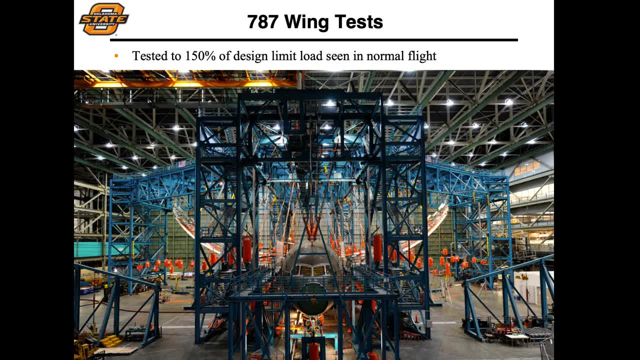 testing and verification of the structural design is really the most critical part of the overall aircraft design and verification process. so even though we don't talk a lot about the structural design in this, this class, you know it really serves as the foundation if you don't get your structure. 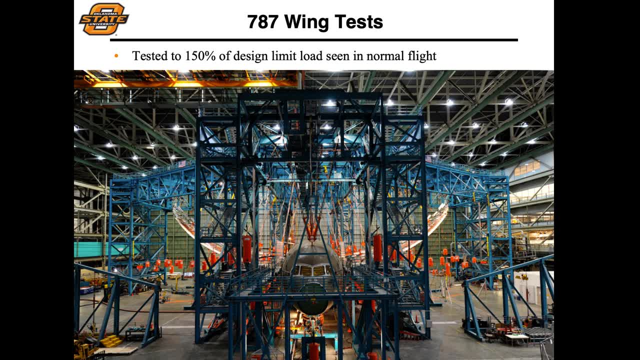 to work, nothing else is going to work on your craft. there's no way that you're going to be able to make your aircraft successful if it is not successful from the structural design standpoint. so here's an example: the 787. again, this is kind of hard to see in this particular 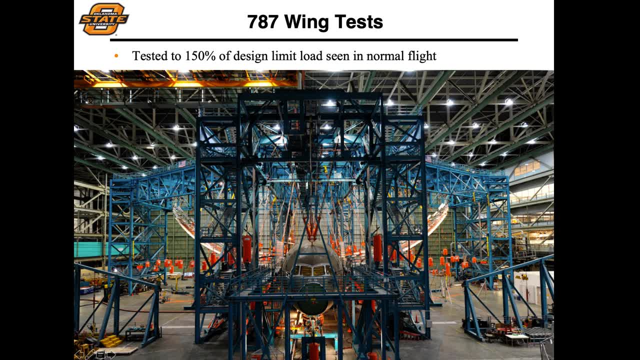 picture. this is our structural test rig for the wings. which will notice is the fuselage right here in the center and look at the wings and so here pointing out the starboard wing on the left side of the picture and our port wing on the right side of the picture. here you can see, for this particular 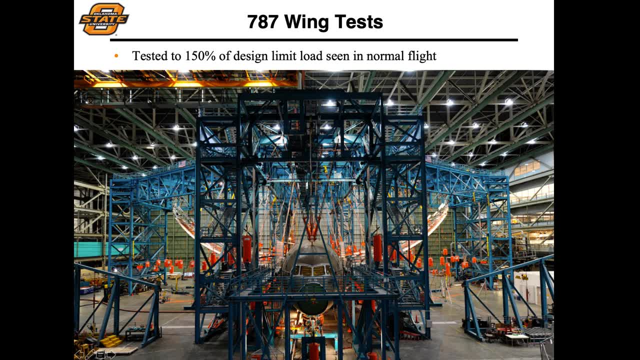 design test, where it's tested to a hundred and fifty percent of the design limit load. so in this case, our design limit, as mandated by the FARs, is 2.5. so they're testing 150 percent of that design limit load to make sure it's not going to fail. so that's. 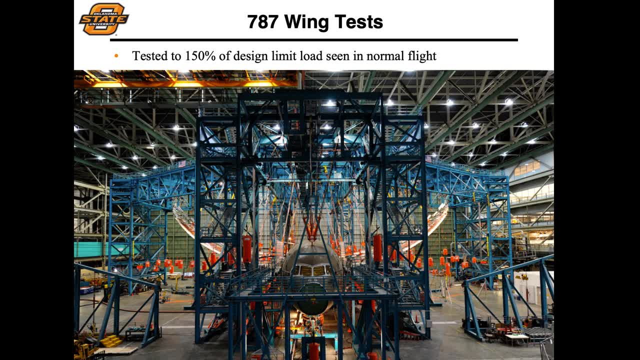 that's the point where you want to make sure your aircraft is not going to fail. if it gets to 151 percent and fails in, that's fine, you're perfect. but you got to make sure that it doesn't fail at 149 percent. so you can see the extreme flex that these wings are actually undergoing and trust. 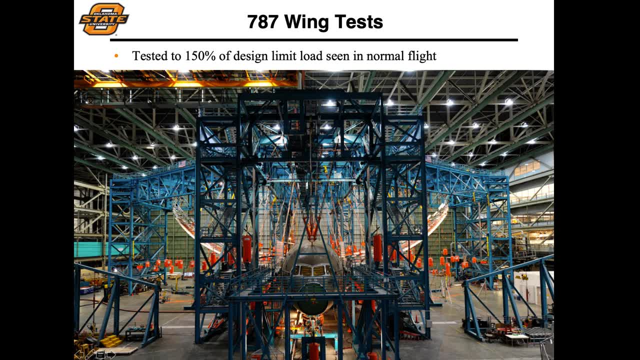 me, if you know you looked out the window and saw the wings undergoing this type of deformation. you'd never notice because you'd be screaming along with the rest of the passengers based upon whatever the aircraft was doing to put the wings in that extreme loading scenario. so I'm not 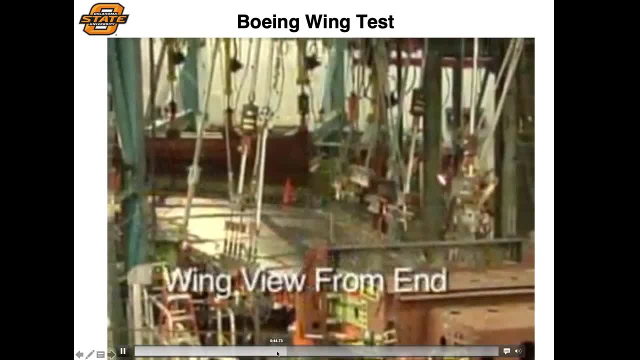 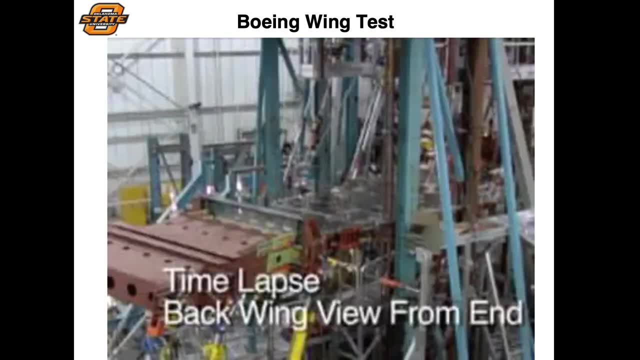 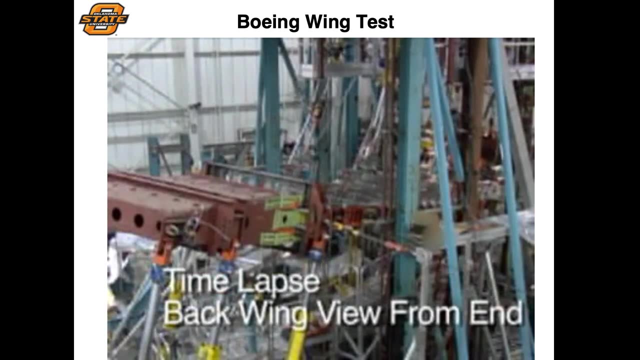 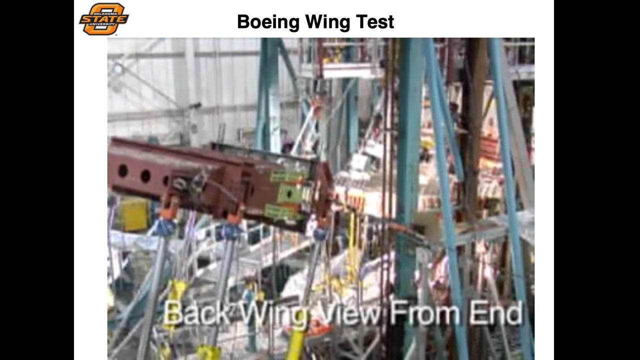 going to be forgetting that. again, that's the wing brake test. so there's a wing toll level process at reference, right below the flap against the wing feed, and, yeah, the g-plug is Devon. that's привow value is calculated at one of the landing stations in the carrier. so this is the wing brake test as it's going through this process and again, so the jig that is built around this to push the wings through this simulated loading scenario, so that way you can measure the load and evaluate the point at what it exactly brakes at thatöhundred one50 percent or greater mark, and you'll see this snap here in just a second, as it 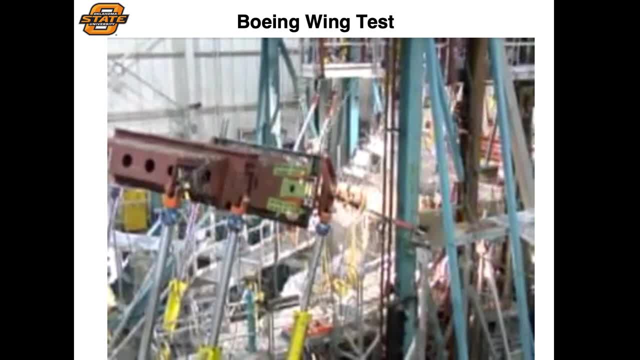 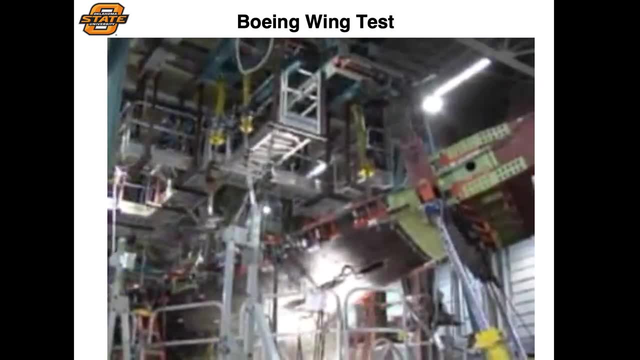 Kabir Periwalier. hundred fifty percent design point and essentially breaks. and keep in mind that this is a partial composite wing design, so you know doesn't just necessarily snap off. there's a failure in it. there's a lot of energy now that's stored up in. 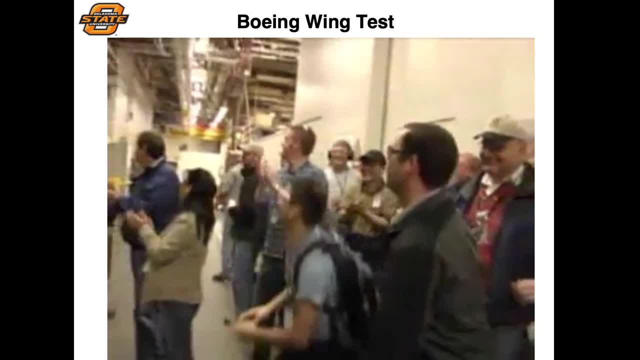 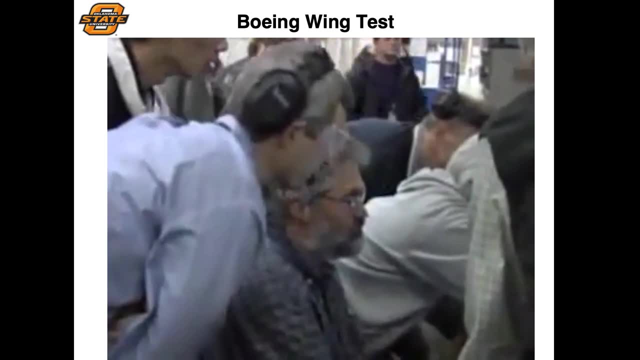 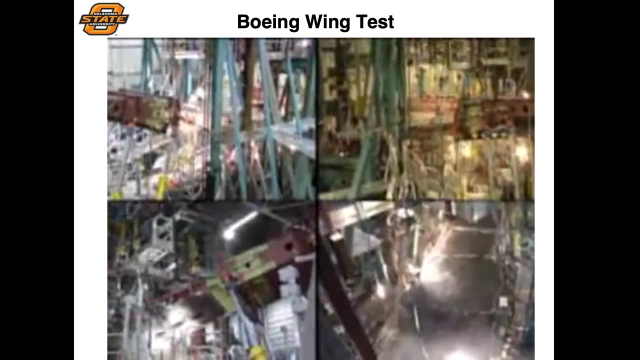 these wings and you can see how it essentially breaks. and two, and you know they're all happy because it failed, but it failed where they expected it to fail, which is exactly what you- you want from a testing standpoint is you've already gone through the process of designing this and you know where that's going to. 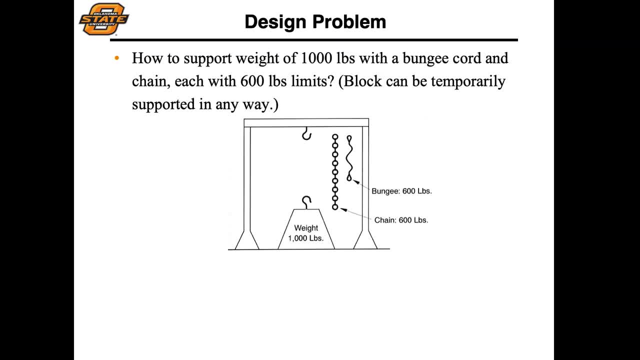 fail at, and so you're validating your predictions. so, as an example, when we're designing an aircraft, we'll typically see, as I mentioned before, multiple load paths. so one way to think about this is you might have an internal structure of your aircraft that's carrying part of the load and you'll have that. 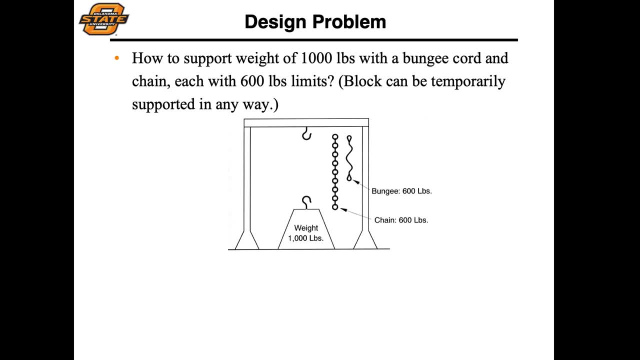 designed in a certain fashion, with certain materials, and then you'll have a skin which is also going to carry some of the load, but it's going to be fashioned in a different manner and it may be made out of or manufactured out of other materials, so they're each going to have separate properties. so imagine this from: 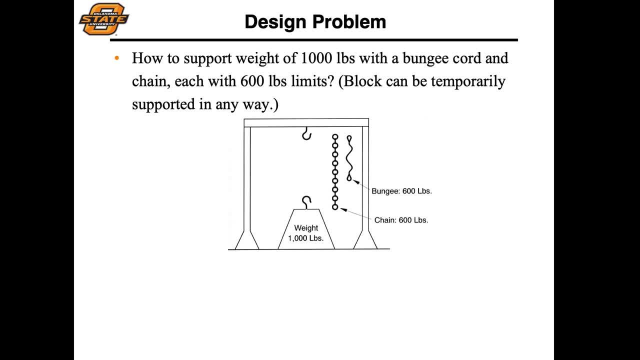 the standpoint where, let's say, we want to carry a load of a thousand pounds but now we're using two different materials that each have similar load carrying capabilities but they have very different material properties. so one is a chain which has very little stretch or strain capability associated with it, where another is a 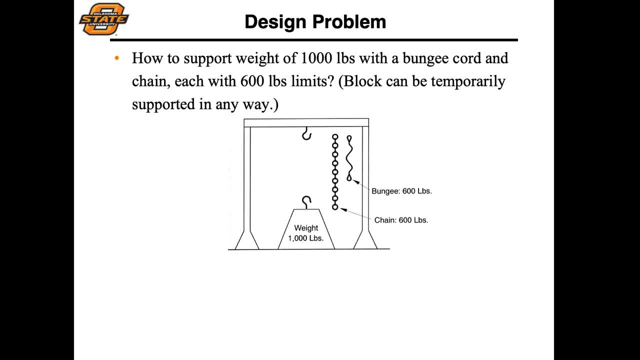 bungee, which has a very large strain capability associated with it. so how would you then deploy both of these in order to be able to carry that load? so you would design this in such a way that, if you want to carry that a thousand pound load limit, 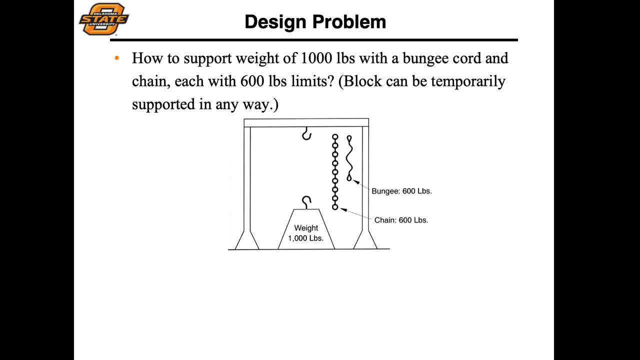 you know, you would essentially be able to design this around one system, reaching or straining or stretching up to a point where it would carry your design load which is going to be less than that overall load limit of 600 pounds for that individual component. and then, once you have that in place, then you can. 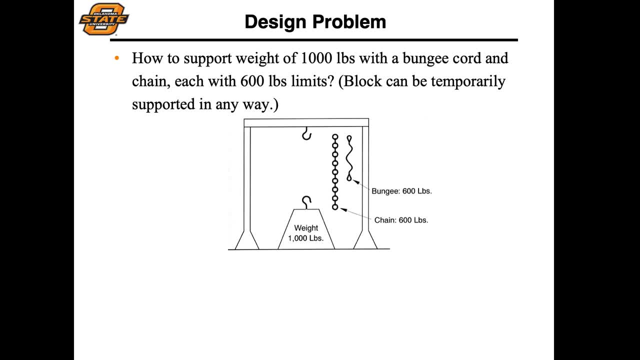 couple that with the other material that you have that has a much lower strain capability associated with it, And now both of these materials would then be working in tandem, and this kind of basic philosophy is how we approach a lot of our design requirements for aircraft when we start putting. 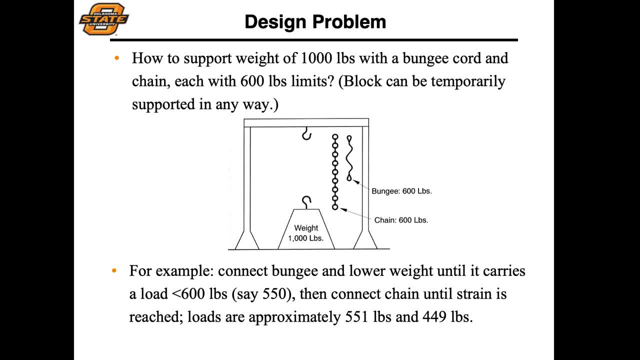 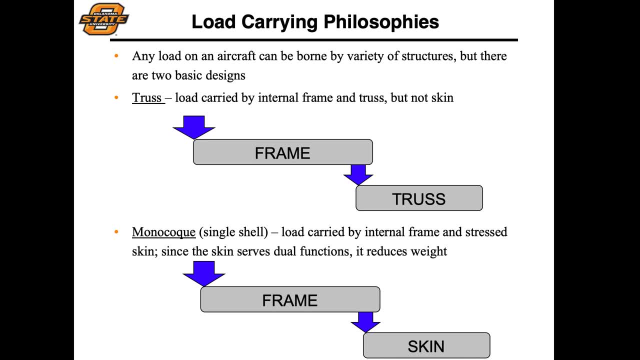 these different pieces for our aircraft together. Now, as part of this, again, we can think about this from a philosophical standpoint and how we're going to carry that load for our aircraft. Now, as part of this, again we can think about this from a philosophical standpoint and how we're going to carry that load for our aircraft. 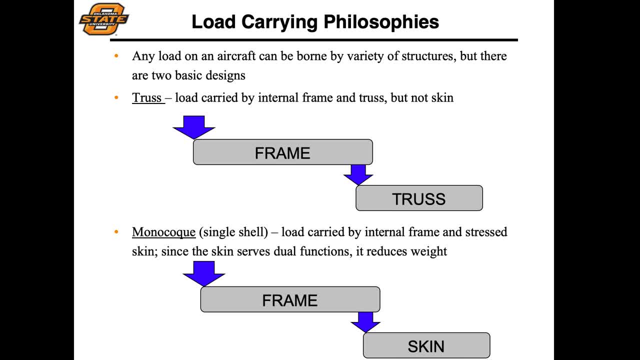 Now, as part of this again, we can think about this from a philosophical standpoint and how we're going to carry that load for our aircraft design. There are really two basic structural design philosophies or structural design configurations. One of those is you can think of as a truss. 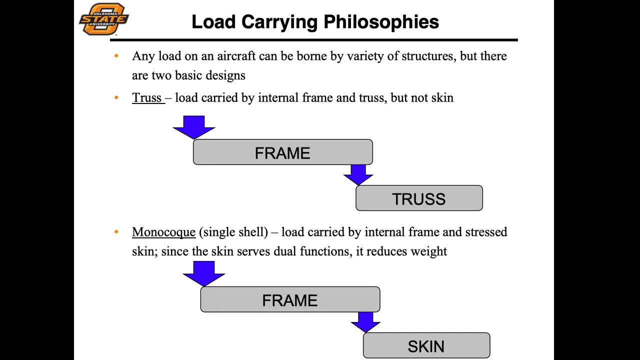 design where you have your load carried by an internal frame and a truss but none of that load is carried by the skin and you can think of this as very traditional in our, you know, wood with fabric-doped early aircraft designs where you have a frame and truss system. 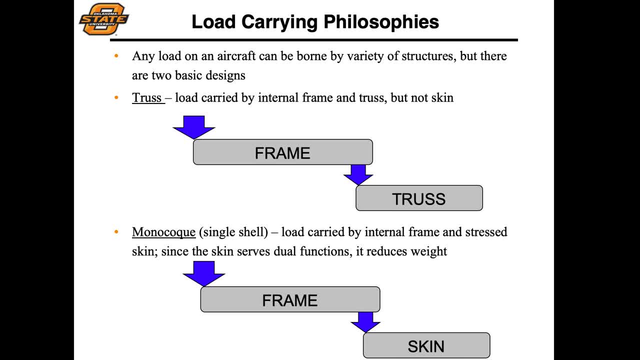 and the aerodynamic loads are really just immediately transferred from the skin directly to that truss and they don't carry any of the loads themselves. A more modern approach is the, the monocoque approach, where you have some of the load being carried by the internal frame but you also have a 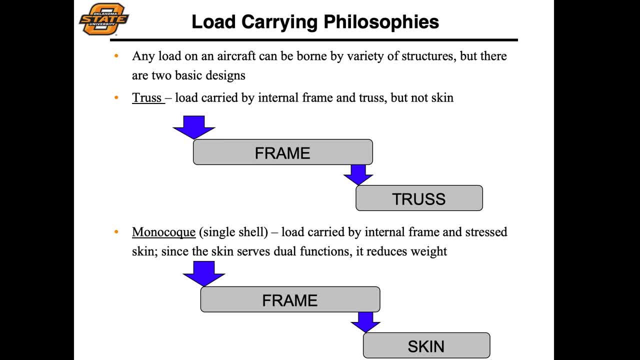 stressed skin, So that stressed skin serves dual functions. You know, it's not only transmitting your aerodynamic loads directly to your internal frame, but it's also carrying some of that load as well, and in this case, if you follow this particular path, then it usually leads you to a lower 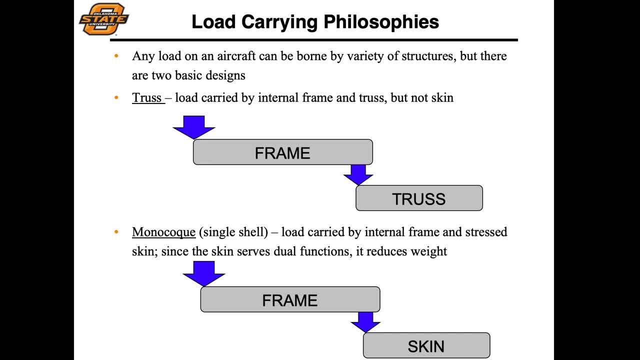 weight as well. So it's a weight saving philosophy, using this monocoque process, And, for those of you who will be in Speedfest next year, this is essentially the approach we use with composite wing aircraft, or we have, you know that, composite skin carrying part of the load in addition to 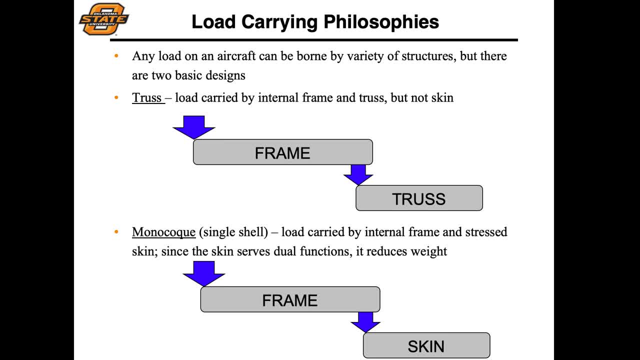 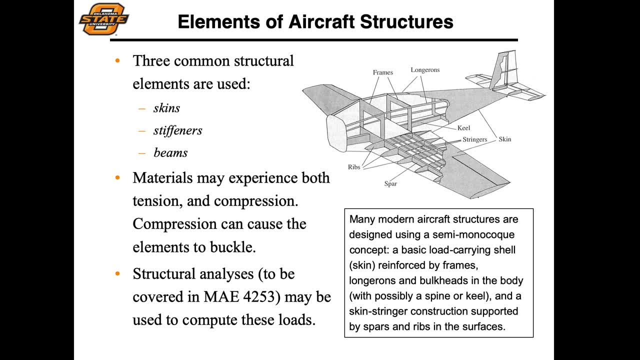 the internal frame that's carrying portions of the load as well. Now there are many different structural elements that we'll have across an aircraft. you know all kind of with unique configurations, and we're not going to go through all of them, but you have primarily three common structural. 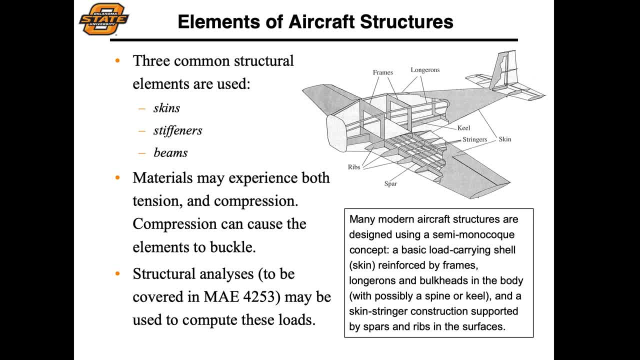 elements: The skin, as we mentioned, stiffener elements which provide a stiffening capability to different components of this skin, and then those internal truss components, primarily made up of different beams, And you'll notice that we have kind of very specific elements that we'll refer to. In wings, for example, we'll primarily have spars, which 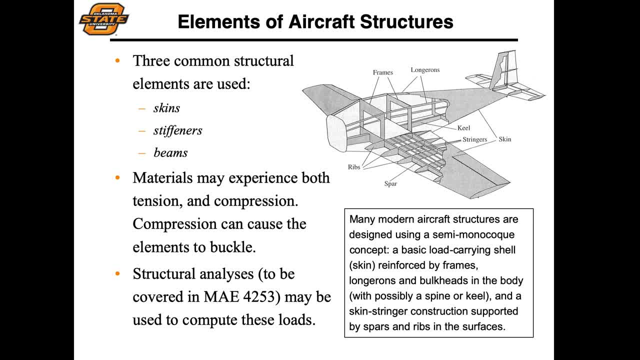 run along the span of our wing, and then ribs, which run along the chord length of our wing. So the ribs will be carrying loads that's transferred from the skin directly to the ribs and then that load is transferred from the ribs to the spar and then the 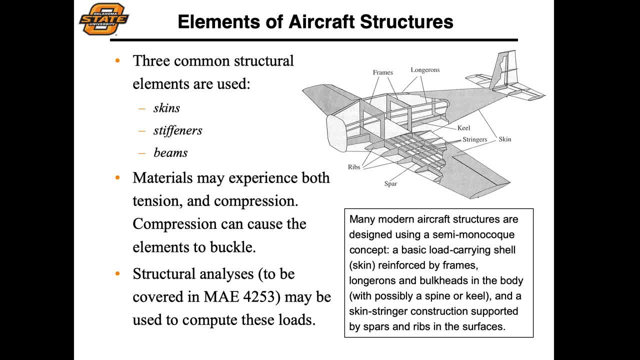 spar transfers that load directly through the wing box structure to our aircraft fuselage, And the fuselage itself will usually have frames which run along the stations from the nose to the tail of their aircraft and then we'll have long runs which run down the axis of the aircraft. Sometimes we might have a keel which is. 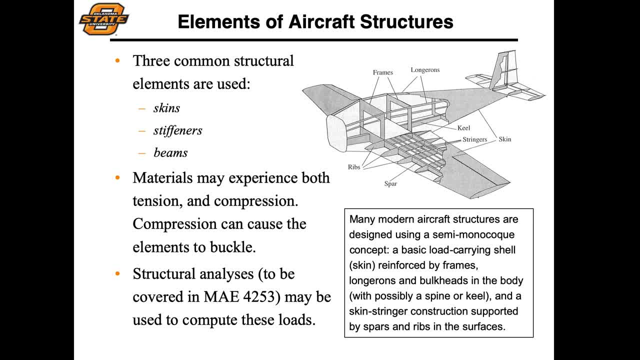 typically going to be loaded, located on the lower side of our aircraft that will carry main loads for the fuselage, but also loads from the wing and the gear. Now, all of our materials in our aircraft may experience both tension and compression. Think about what the load is happening on the wing as it goes from positive g-forces or positive load. 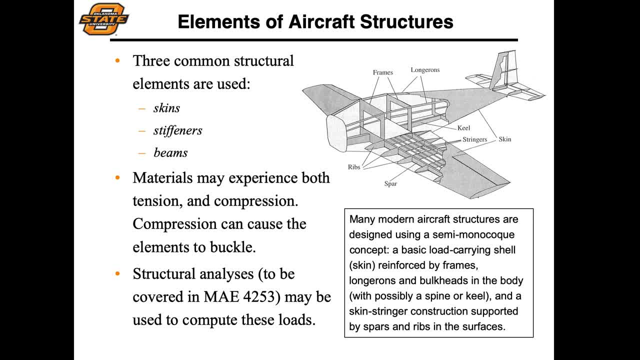 factors to negative load factors. So at some point you'll have compression on the upper side, tension on the lower side and as you reverse those load factors the tension and compression will swap from the top to the bottom. So you will analyze or utilize a lot of structural design and 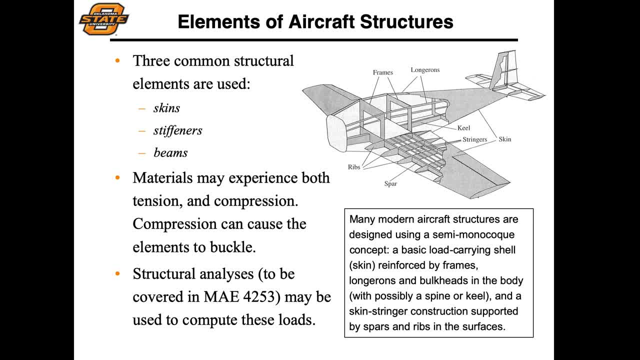 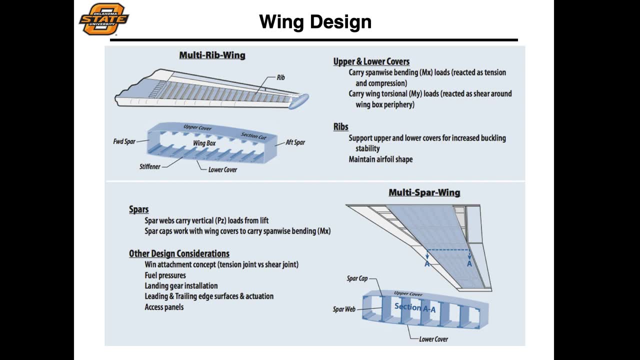 analytical approaches, We'll be able to go through a process of analyzing the loads and then designing around that. Now, as examples of the wing designs, you can have multiple ribs and multiple spars, and that's going to be typical configurations for most modern aircraft wings. We'll use many different ribs. 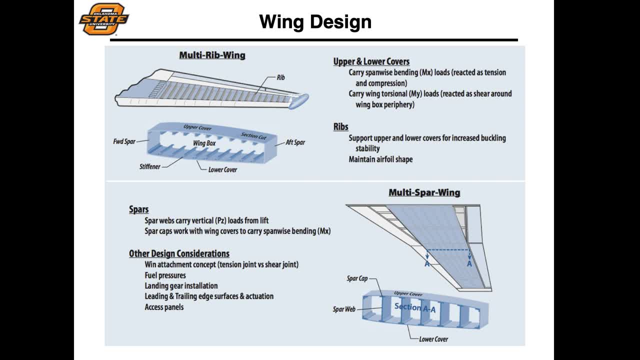 along with multiple spars, Typically at least one spar located at the quarter cord and a smaller spar located at the three-quarters cord, But you can use many different spars across the wingspan as well, And there'll be lots of different ways that you can combine these together to provide weight savings. 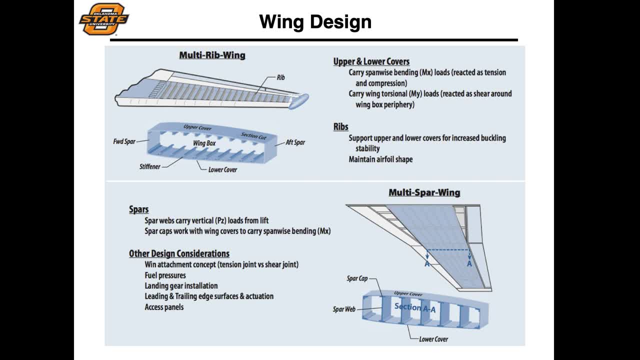 for your aircraft while still being able to carry the same load, Primarily depending upon how you utilize the ability to minimize your weight while maximizing your cross-sectional moment of inertia. So you really want that capability to transfer those loads from the cross-section along the length to the fuselage. 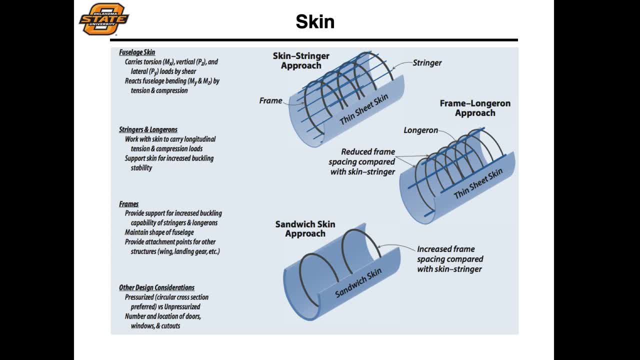 portion of your aircraft. Likewise, with the skin, you can have lots of different ways that you can design the load-bearing capabilities. Now for most aircraft- modern aircraft- these are typically going to be pressurized. Not always, You know. lower altitude aircraft, like general aviation aircraft, will usually not be pressurized. 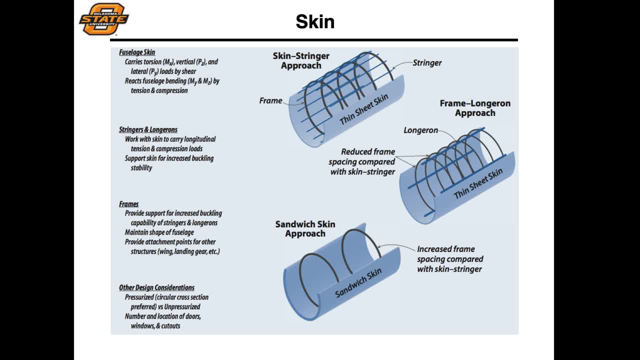 But anything that's typically going to be over 15,000 feet in terms of its flight capabilities- including, you know, modern airliners and other transport aircraft- are going to be pressurized. So in this case you can think about that fuselage as a pressure vessel, and then you can. 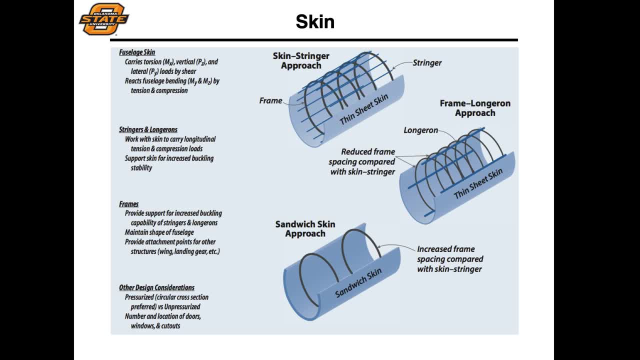 use the same pressure vessel equations that you're already familiar with to go through the process of designing the load carrying requirements and looking at the hoop and axial stresses acting on that pressure vessel. And once you know that, then you can understand the process, that which you'd go through to reduce. 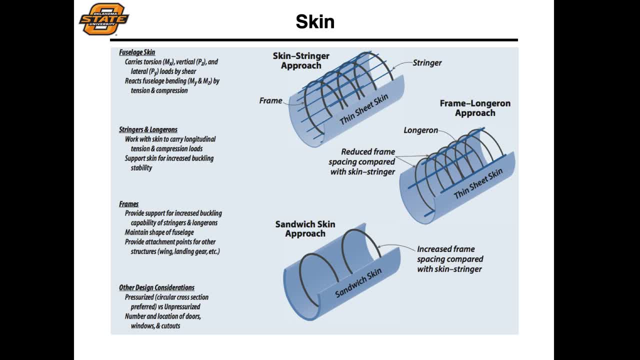 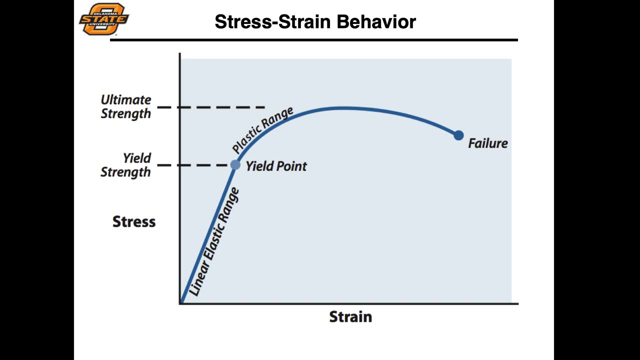 the weight of that pressure vessel to carry that same load by using things such as long runs or stringers or hoops to be able to carry some of that additional load. Now, as you recall our traditional stress-strain behavior for materials, as we're deforming that, 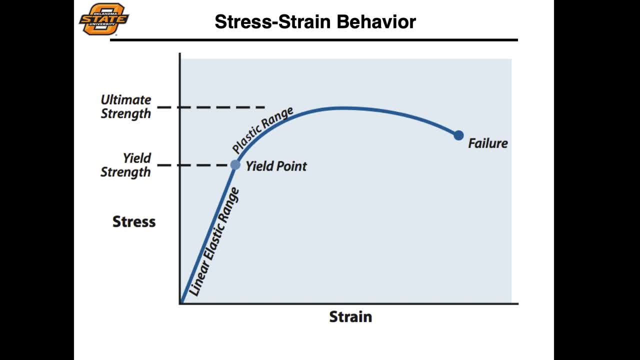 material. increasing that strain will have a linear region where our stress is increasing linearly with that strain or deformation until we get to some yield point where we'll then experience a non-linear plastic deformation regime until we get to the point where that structure fails. Now this behavior is highly dependent upon the individual material. 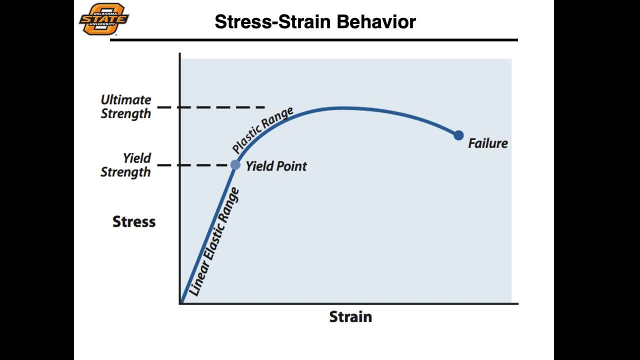 structure Characteristics, the behavior, in particular of where that yield point is at the plastic range, and then ultimately, that failure. That failure point can be much closer to that yield point than is shown in this particular conceptual figure, for example, or it could even be farther. 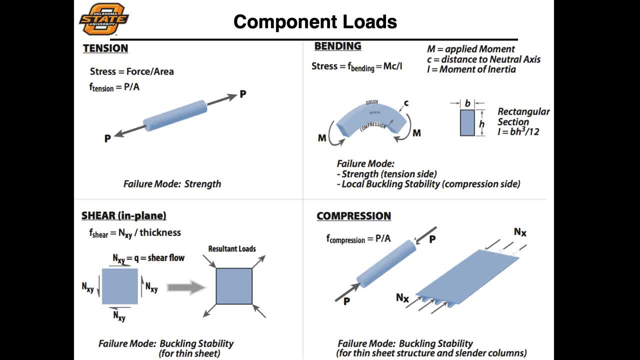 away Now to analyze this individually, we have to go back and look at the individual elements and the behavior of each one of those elements, In particular, looking at our tension and compression forces on those individual components, as well as bending and shear forces. Again, this is going to be in more detail than we need to go. 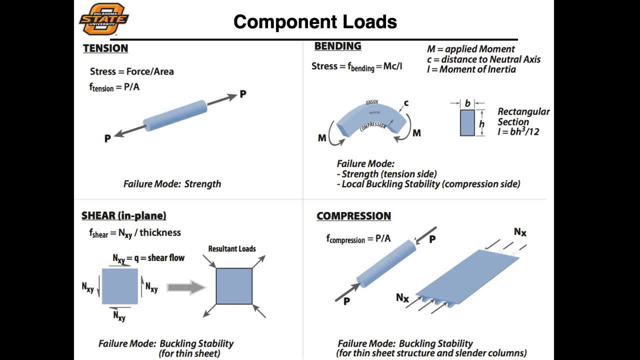 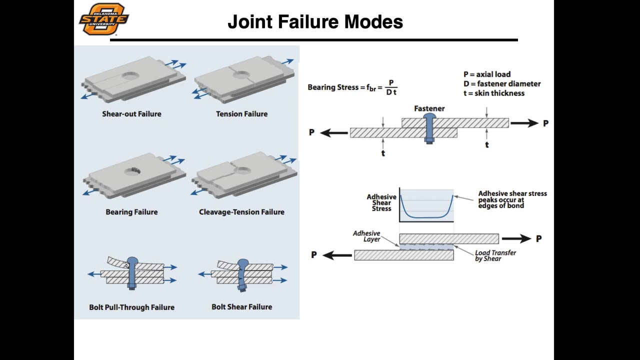 into. but since you're already familiar with these components and these different behaviors, as well as the material properties that you've taken in other classes, it's now just a matter of taking these pieces and putting them together. Now, obviously, we're going to also have to consider how these loads are being transferred. 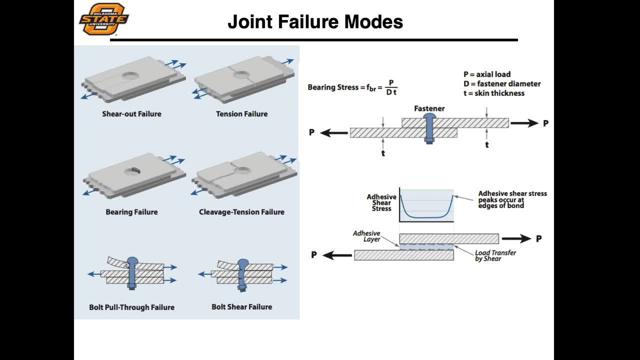 through joints, as we're connecting different pieces together and think about how those loads then are being transferred from one component to another component, And it's usually when we see failures. it's pretty common to see the failures, uh, within these particular joints, because these are going to be the regions of your 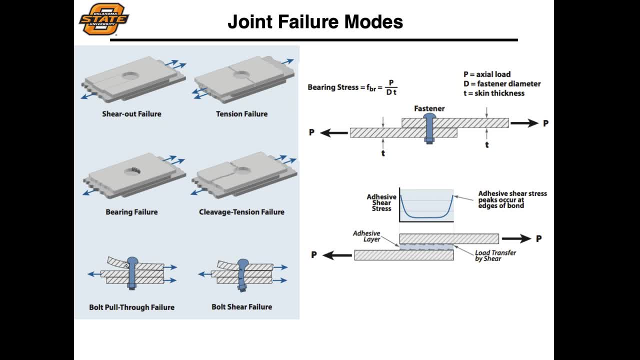 highest stresses. Whenever you're putting a hole in a material, you're obviously going to have stress concentrations uh located near these holes in your material, as well as a greater propensity to have uh critical material uh deficiencies or defects within. 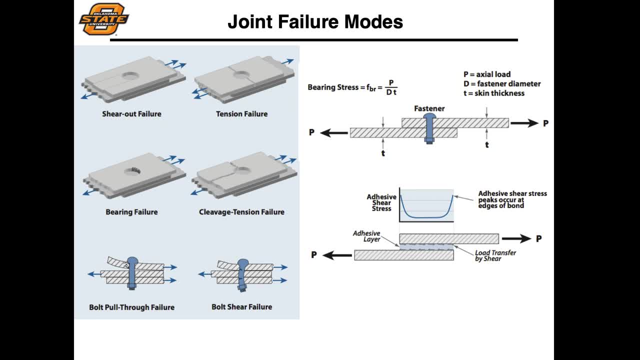 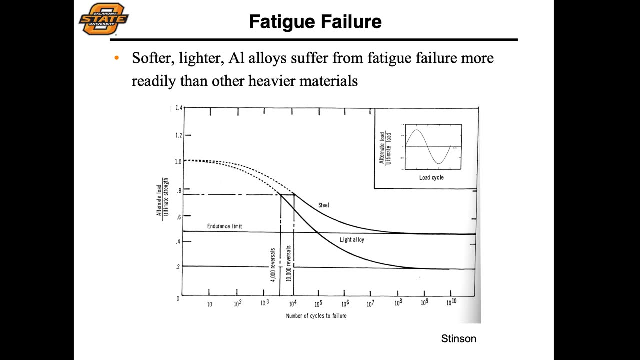 these particular areas. So you might have a crack, and that crack would then propagate, uh, under that stress concentration, and then that might result in a failure. Now, what we often see in aircraft failures is the impact of fatigue, and so, rather than 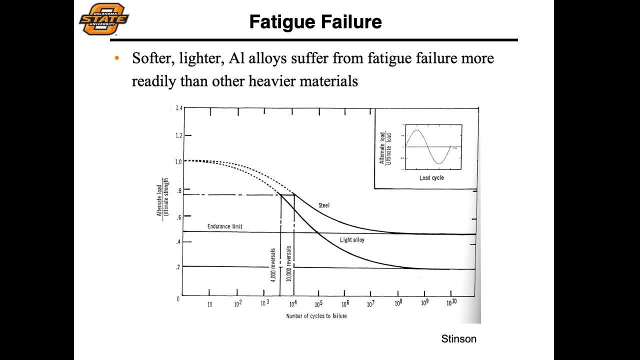 a failure, uh being immediate. what we're going to see is that material uh start to degrade over time as it goes through cyclic loading. Think about this in the context of of your wing, as it becomes loaded and then unloaded, loaded and then unloaded For every. 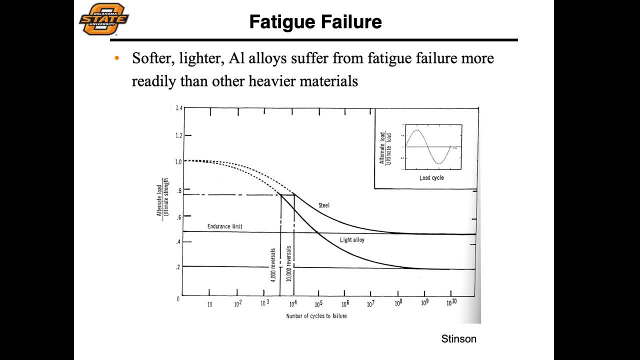 flight that it goes through. it goes through this process of being loaded to extremely high loads and then unloaded back again repeatedly, perhaps multiple times per day. So you might have this process happen, happen a thousand times or more a year. So you obviously 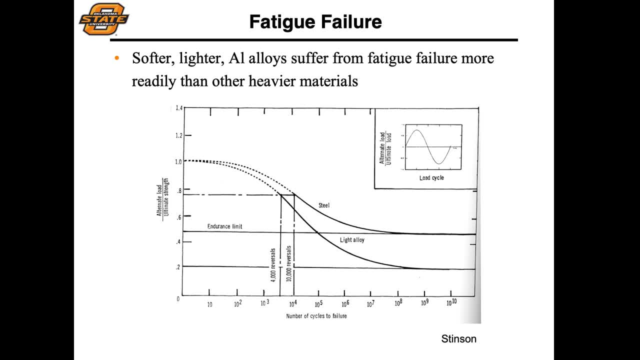 end up with a lot of cyclic fatigue. uh, possibilities, Uh, the best common um day example that I can give is a is a paperclip. Take a paperclip and you think about: well, I want to snip this paperclip in two. Uh, you know, you go. 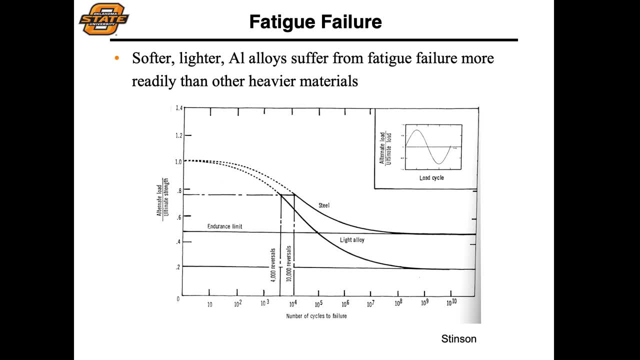 to. you know, get a set of shears. think about the energy that goes into that to be able to snap uh. you know that thin paperclip uh in half. But if you want to do that easier without going through the process of using a mechanical uh, implement uh, then just. 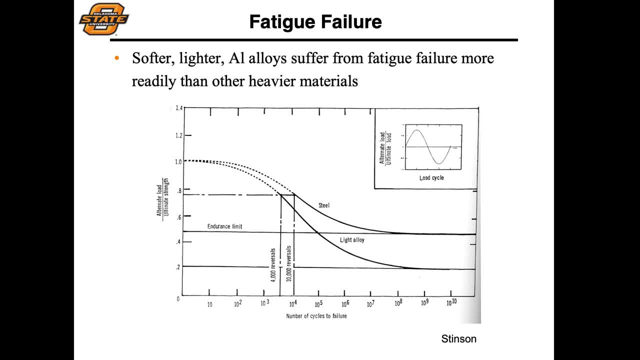 do some cyclic loading, Typically in about ten cycles, uh, you'll be able to take that paperclip and fail it. Uh, so this is very similar to what you'll see with aircraft As you go through the process of cyclic uh, uh, uh loading, uh over and over, you know, repeatedly, uh, you're going. 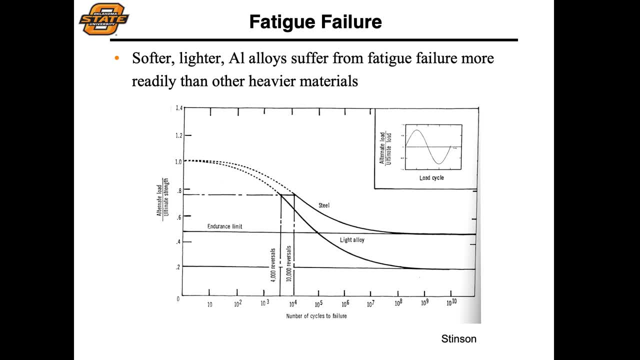 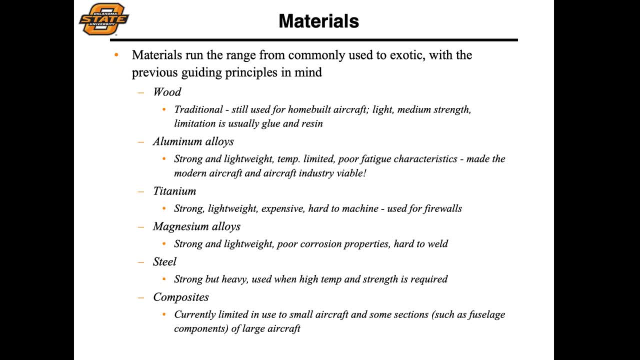 we're looking at aircraft that might be designed for very extreme environments. you know, maybe such as a space shuttle type of design or a fighter aircraft. you might be willing to pay more if we're really able to push the capabilities of those individual materials. So we're going to look. 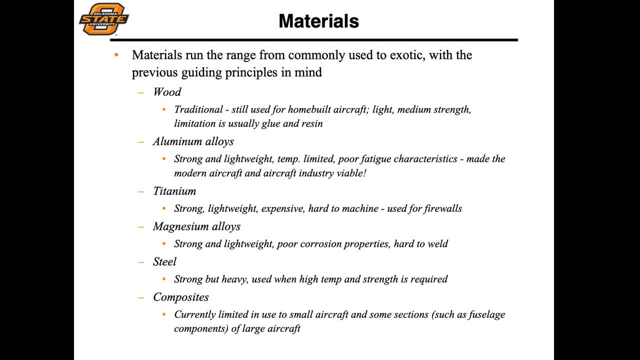 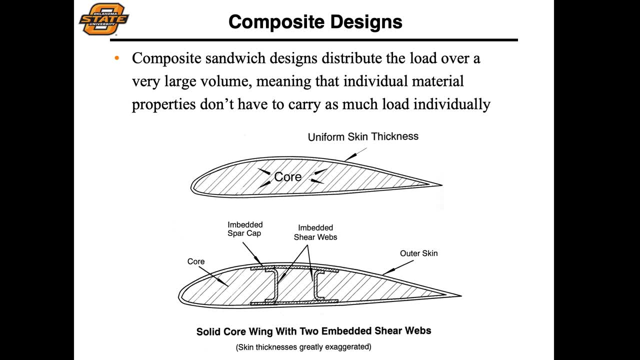 at a range of different materials as part of our overall trade study. Now this includes composite materials. When we start looking at composite materials, that allows us to look at other options as well, rather than kind of traditional overall designs, particularly sandwich configurations, where we can distribute loads over a much larger volume. Now, one thing that we had to consider: 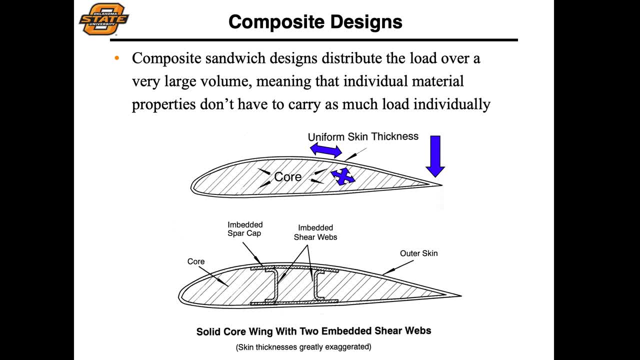 when we start looking at composite materials is these are sometimes going to be more difficult to predict, And so, in this case, we're going to look at composite materials as part of our this case, we may actually be looking at a lot of empirical models for our composite materials. 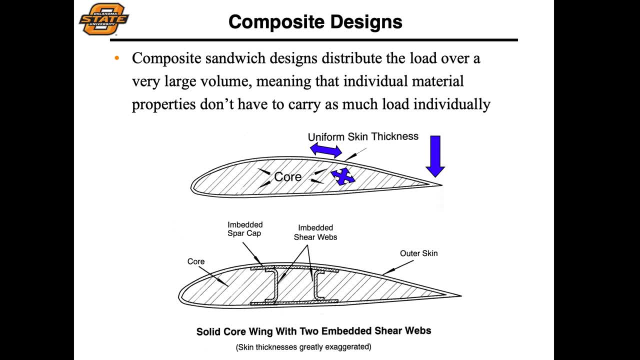 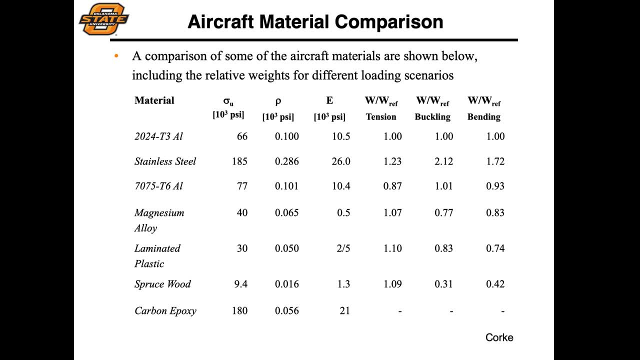 rather than looking directly at traditional analysis. Now, primarily, we're going to be looking at, you know, things such as density, yield, stresses and relating those back to a reference material. In this case, we're going to use the most common material that we'll typically 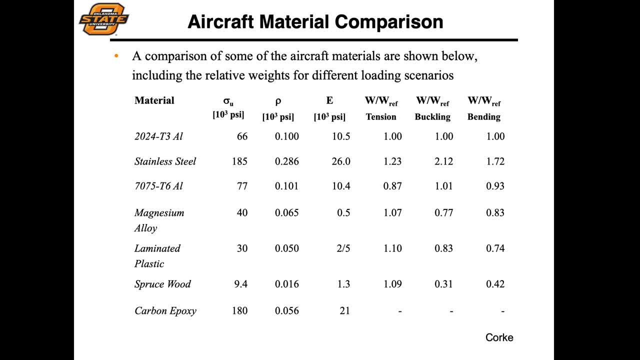 see for modern aircraft design, which is 2024 aluminum. So that's going to be our baseline, both in terms of our tension, our buckling and our bending loads for our aircraft. And you can see from different materials here that we have a wide range of different configurations, but they're 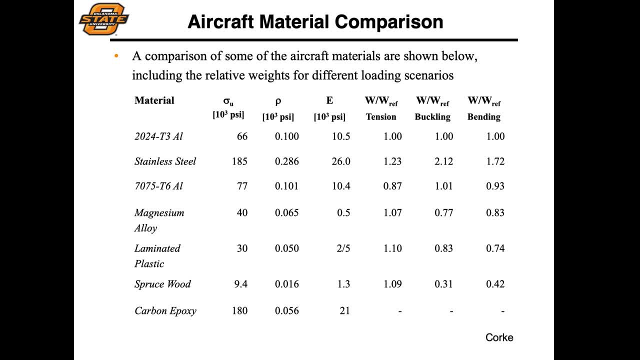 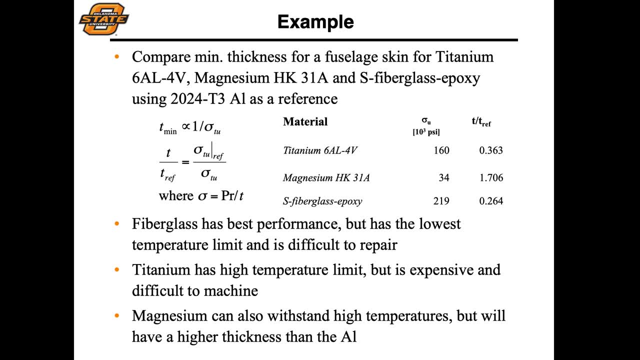 all fairly closely benchmarked to those particular design elements. So, as an example, we can compare a minimum thickness for fuselage skin Using titanium, magnesium and fiberglass and comparing it back to that 2024 aluminum as a reference material In this case, each looking at the stress and then the required thickness of 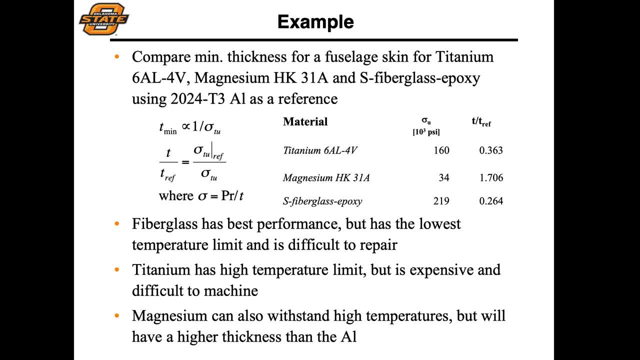 that material to meet those same pressure vessel requirements and compare both that overall stress as well as the resulting thickness, The fiberglass has the best performance, but it has the lowest temperature limit, difficult to repair and also difficult to work with. So that, may you know, rule it out. depending upon the types of 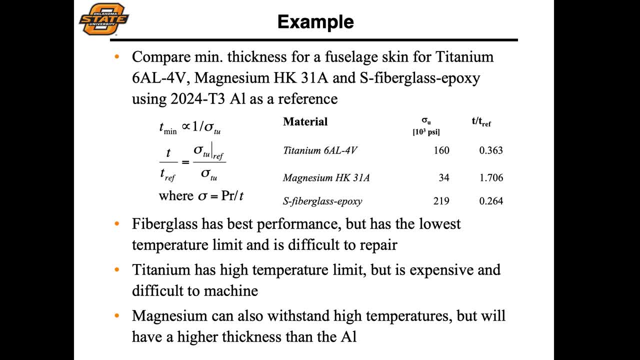 environment that we're looking for. Titanium has the highest temperature limit and a performance comparable to that of the fiberglass, but it's also very, very expensive and difficult to machine. We can see the magnesium can also withstand high temperatures, but in this case has a much higher. 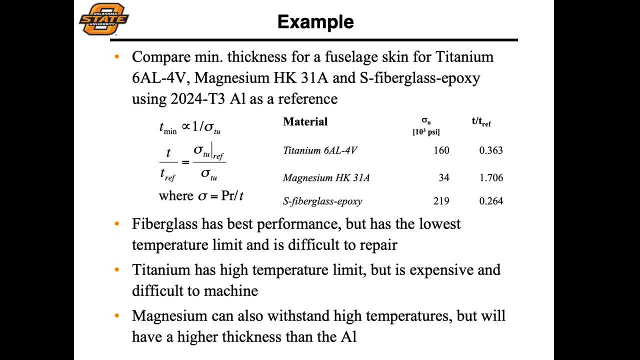 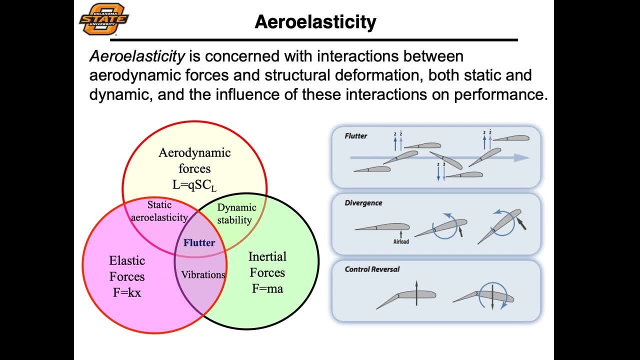 thickness than the aluminum does, and that's going to have a large impact, then, on our aircraft design. The final thing we're going to mention here is really just as a consideration is thinking about how our aircraft structural design is going to behave, not only from a static load standpoint. 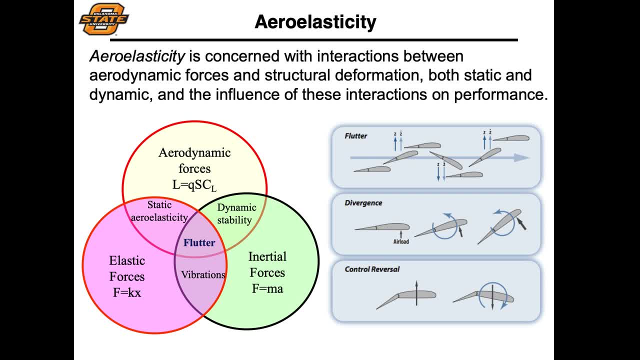 but also from an aerodynamic or dynamic load standpoint as well. In this case, we're looking at the overall science of air elasticity, which is looking at combination of both the aerodynamic forces and the structural deformation, both static and dynamic, and looking at the interactions that are 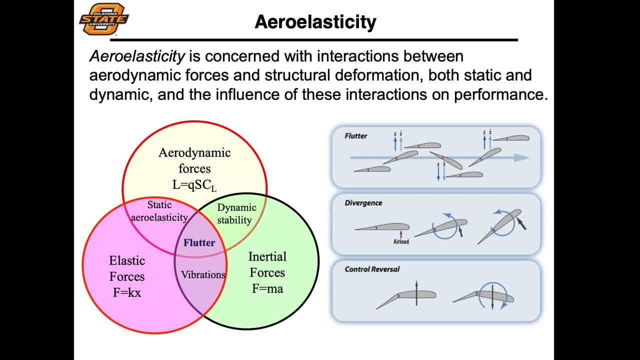 going to occur between these. So when we start to combine all these together, when you look at the aerodynamic forces, the elastic forces that we're going to see from structural deformation, and then the inertial forces, given the weight of our structural design, we can see some really unique things from an aircraft design and